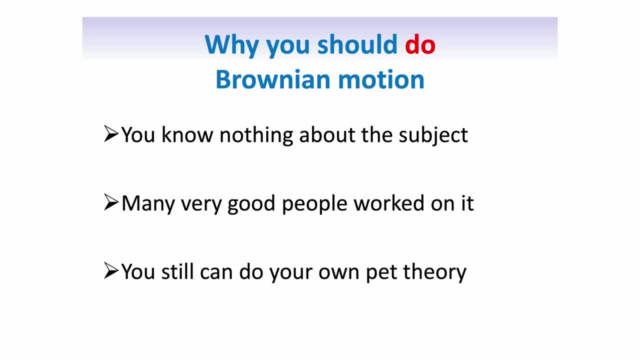 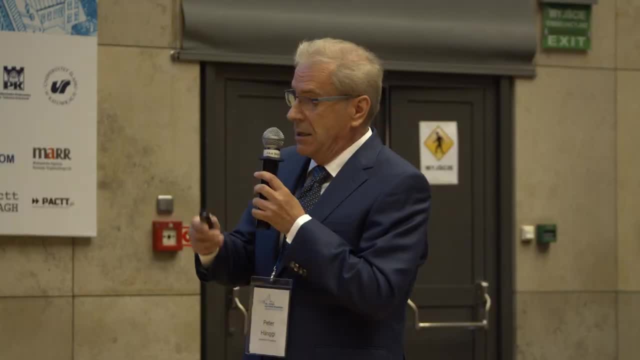 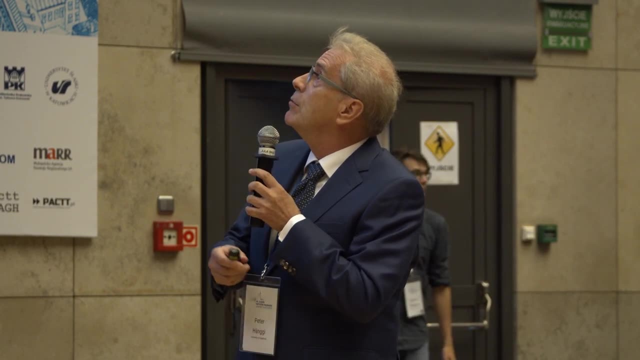 it, Because the fact that so many smart people worked on it it probably means that that is an important topic. That's what I wanted to say before. Okay, now let's see, And I start now with the Brownian Motion. You can read it, Of course. 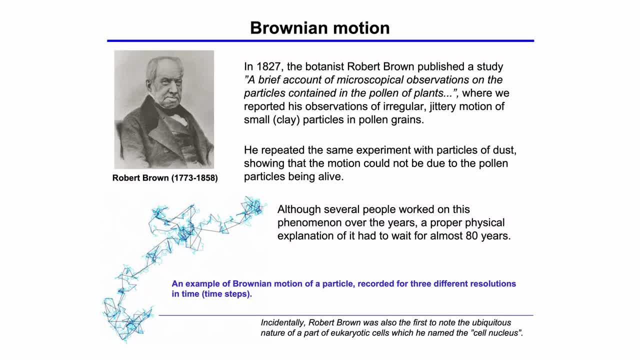 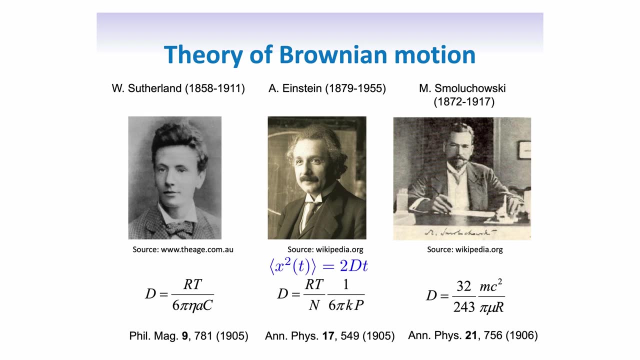 it was invented by Robert Brown when he actually did an early experiment looking at how the grains of pollen move- And this story you know, I go more in physics- It became an important thing. The theory of Brownian Motion has a long history, but it started essentially with. 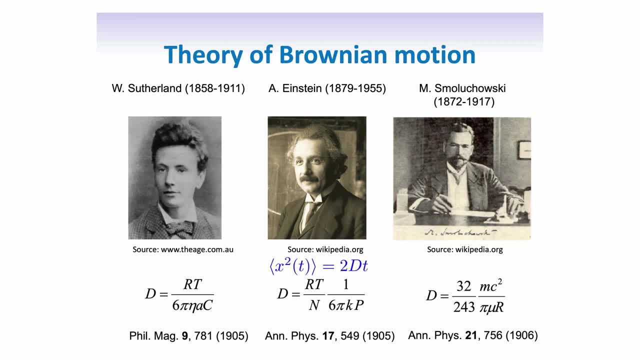 a person which is usually not so much well known. It's actually Bill Sufferland. Everybody knows about Einstein's contribution on Brownian Motion, a 2005 paper, And, of course, Marian Smoluchowski had a much deeper understanding of Brownian Motion And 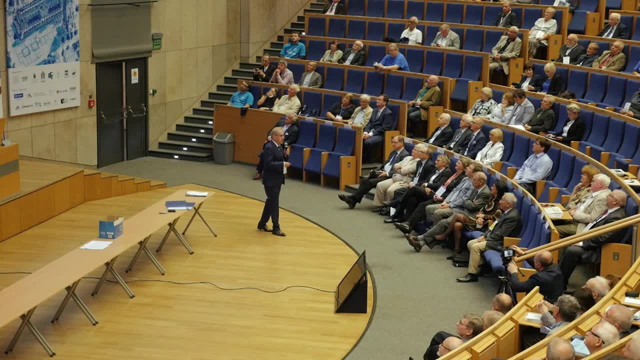 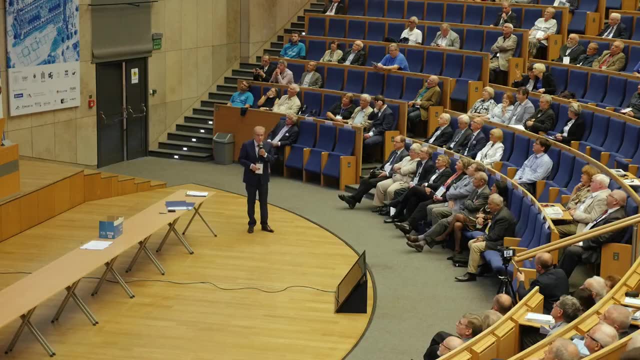 Einstein said he understood Brownian Motion. Well, I actually didn't even know about the phenomenon in the first place. What is a bit interesting to say from a historical point of view, because at that time he was in Bern and we had this group of always four people, which I will. 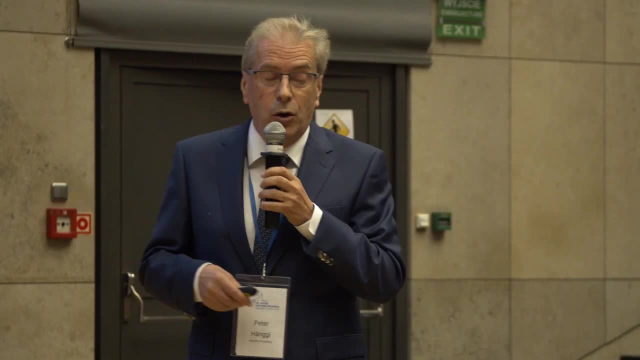 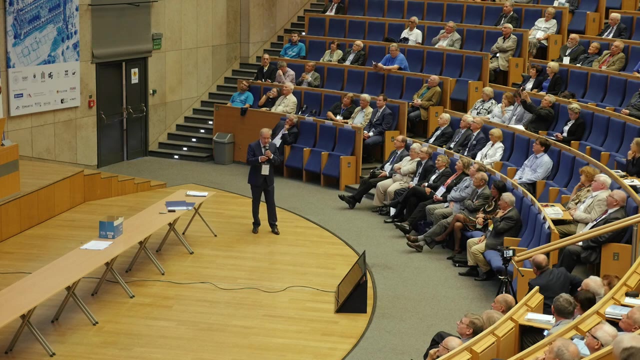 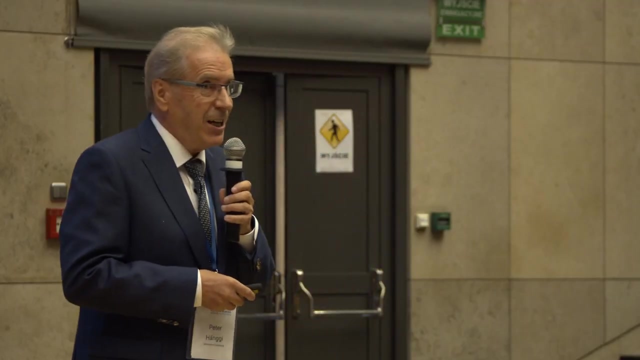 not give you the names because of time- And they studied actually all the papers of this famous- not-so-famous guy, but he should be famous- Bill Sufferland. And, as a matter of fact, what we call the Einstein relation has been discovered and published quite a bit earlier than Einstein. But 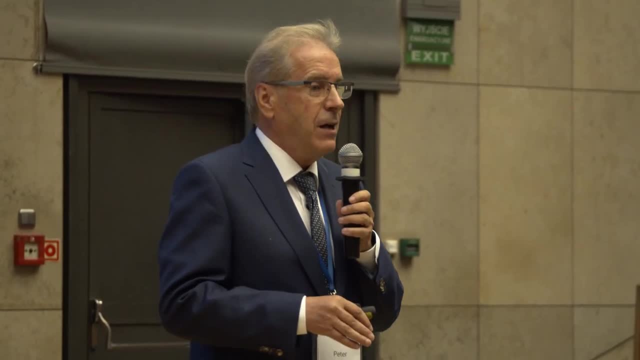 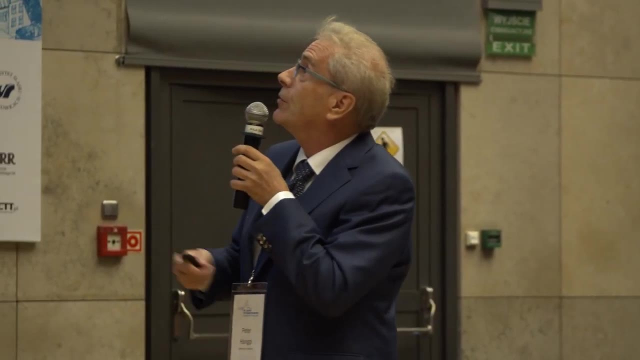 Einstein was a person. He was very convinced of himself. He essentially never gave credit to other people, which is what they did before, And here I have the proof. You find all of this in my homepage. This is actually the text of the Sufferland paper where he balances the osmotic. 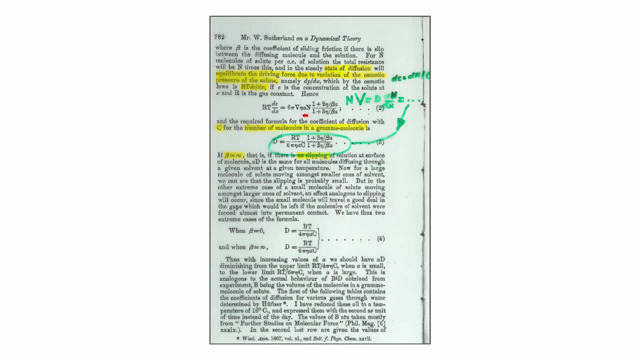 force, the Stokes law force, And then of course, having this relation, it follows immediately that relation here that the diffusion coefficient is given here by the gas constant times, temperature, So R over C is the Boltzmann constant, And he even did the theory here for slip. 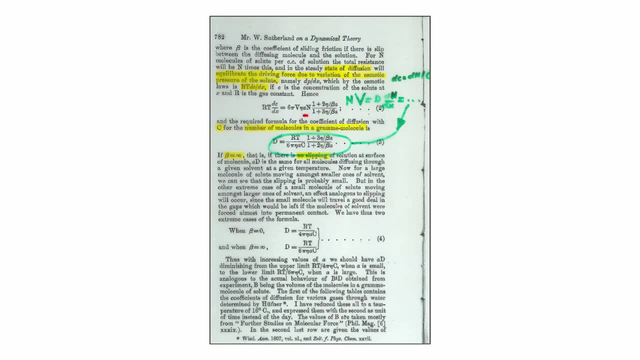 and stick boundary conditions to, so to speak, relate the Einstein relation. But you see, the Einstein relation is essentially already part of here. You see it, all of this is written down in that small, in that paper by Sufferland, which was essentially eight months. 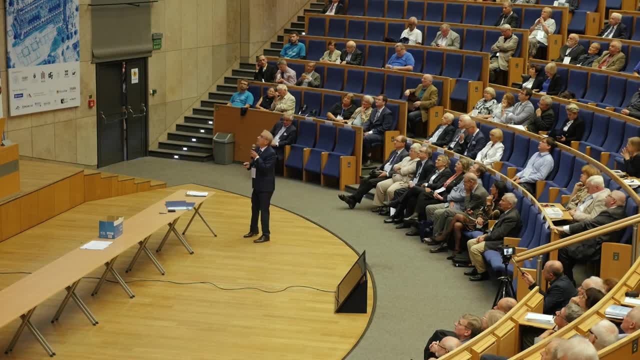 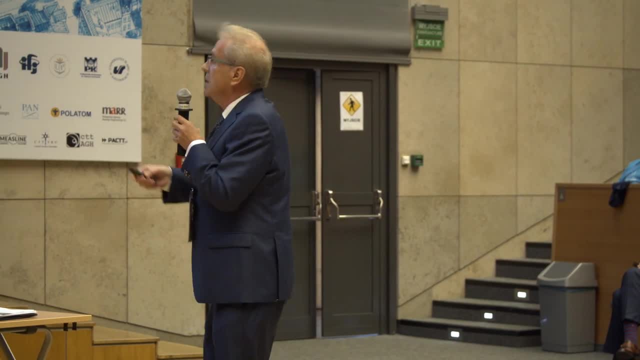 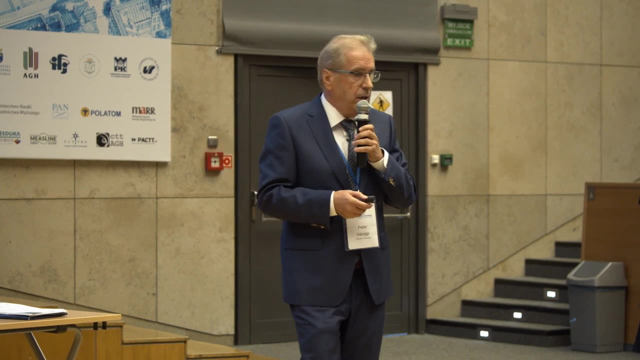 published before even he submitted his work Nowadays, just to advertise this. why Brownian motion is an important subject. I start with maybe the high energy physics and field theory. Of course the path integral formulation is based on mean noise and things like that, And 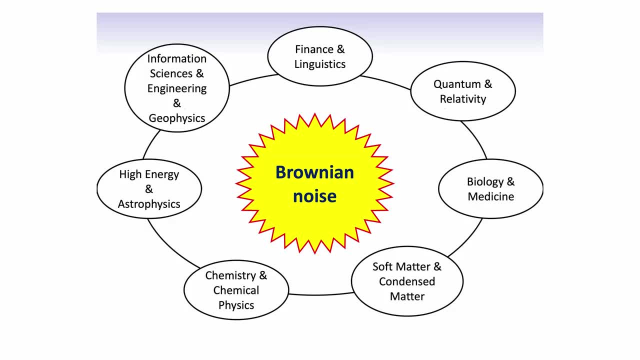 there's a field called stochastic synchronization. Even in finance and linguistics we have a lot of Brownian motion theory Ethos to cast differential equation to explain the stock market development. Of course, chemical reaction, soft matter per se, biology, now also. 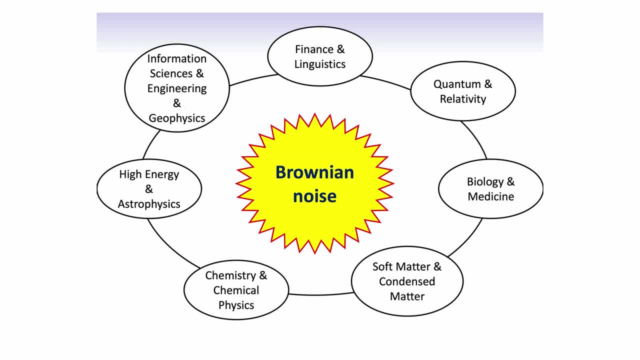 all the time- and information science and geophysics. I will give you some example And a little bit. the problem is actually relativity and quantum relativity per se. I will actually relate to that because I did work in this also- And just another big problem we have. 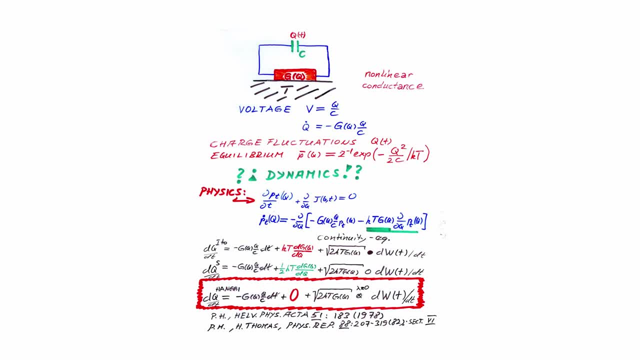 as a physicist, usually we know the deterministic laws. For example, we have here a non-linear resistance, but in contact with a thermal bath, with G of Q is a non-resistant and with capacitance C is a linear device. You know what's the energy is? essentially is a charge. 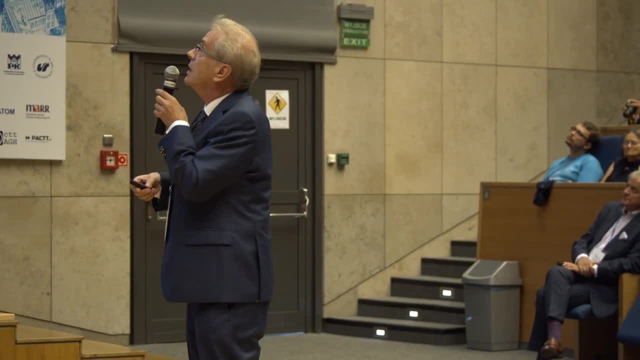 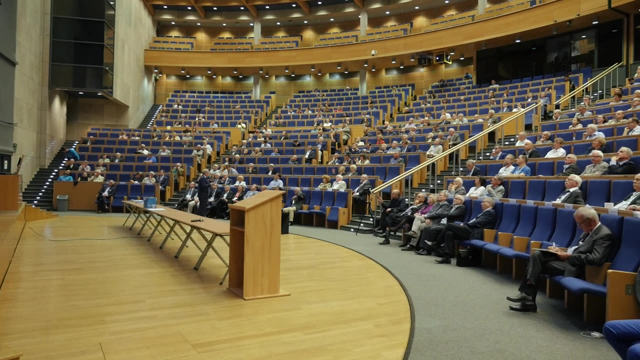 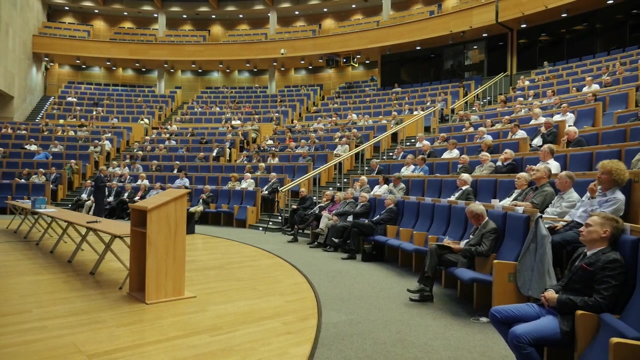 squared over two C. Q squared over two C over KT is the equilibrium distribution which has mean value zero. It's important that this is the correct stationary equilibrium distribution. We have a non-van. it is a Gaussian with vanishing mean. If it would have non-vanishing. 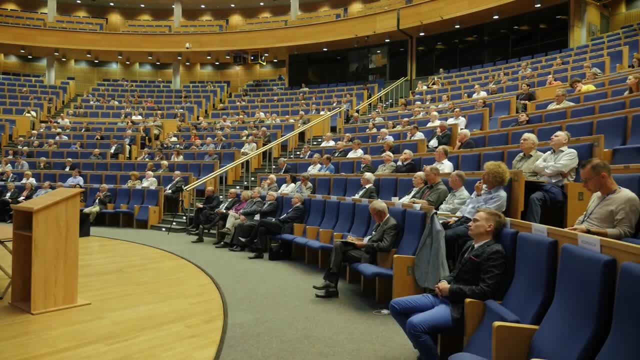 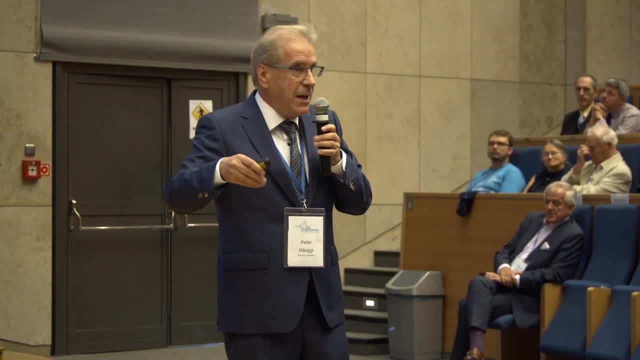 mean you would get a finite voltage across the capacitance and you could build an infinite series and get all kinds from brownian motion. you would get for free any voltage you want. Of course that cannot work, but it's a problem. how to model now fluctuations? because you 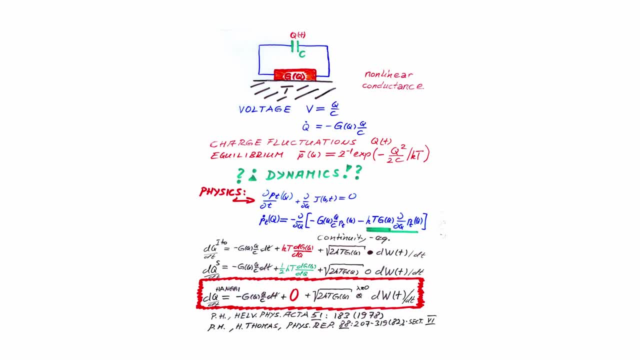 have the deterministic law, on the other hand, the probability theory tells, you have the conservation of charge 0010, And when we have here a nonlinear Einstein relation. and what is important is here, if we have a state-dependent diffusion coefficient or transport coefficient. that's the second. 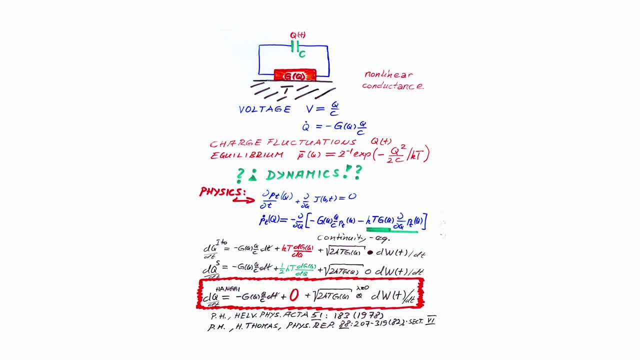 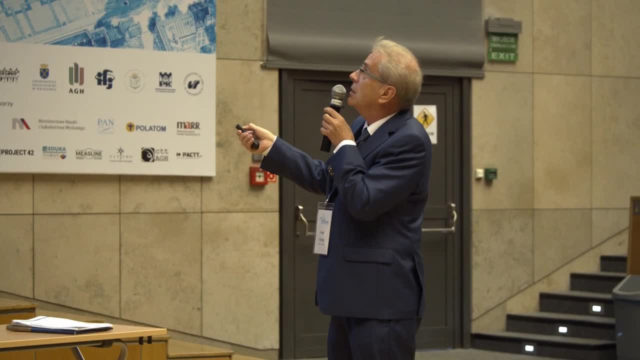 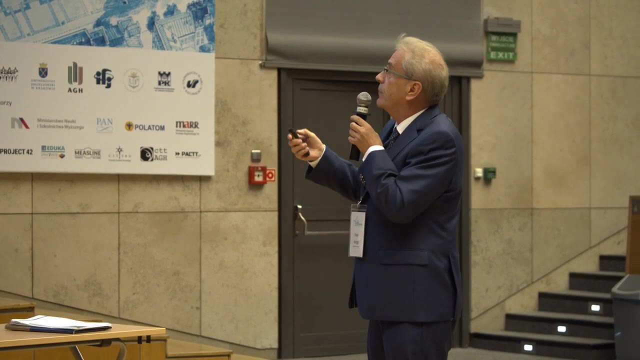 order derivative. the Laplacian is sandwiched in between, in front of this transport coefficient and afterwards. here, as you see. Now, how do you write down now? how do you treat now the fluctuations leading to this probability, to this over-damped Smoluchowski equation? 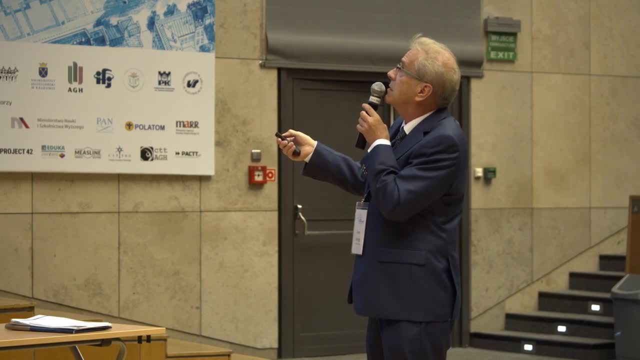 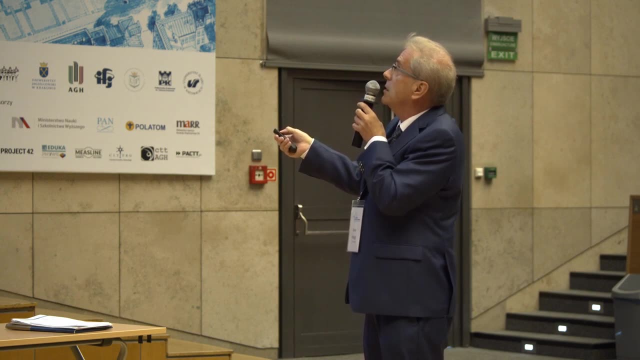 Of course most people would say: you take the Ito rule. you know here's the VAT stuff and you have here the Ito rule with independent increment, which is- I will not go into detail, but here you. but if you do VAT and you don't add here this so-called fluctuate, this part, 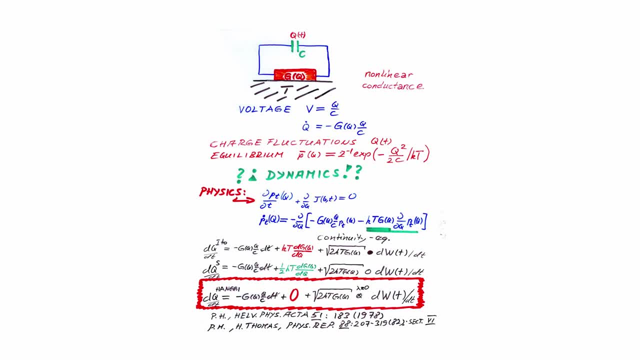 in red. you will not get from this Ito prescription. to this Fokker-Planck equation, Most people say: okay, we use this Dadunovic, because that's, it's so-called, you know, it's considered normal using standard calculus and this uses a midpoint rule. this uses a 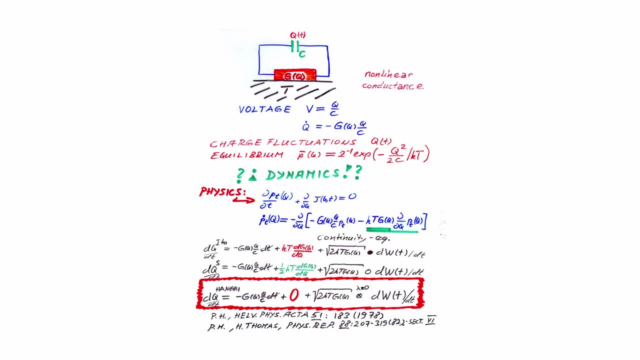 pre-point rule, and then you have to correct it with the green stuff here. in order to get from this interpretation of stochastic calculus to this equation, I put forward, even as a PhD student, a different interpretation. it's called the Hanke interpretation. 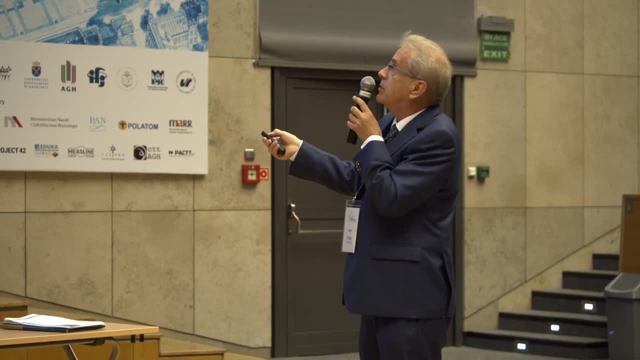 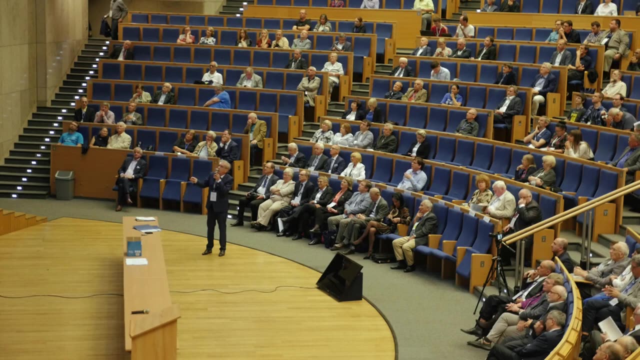 or the transport interpretation, namely I use the post-point in the discretization of the Wiener increment between V of 3 and V of 4.. Okay, T plus delta T over minus V of T. you have to actually look at the post and then you. 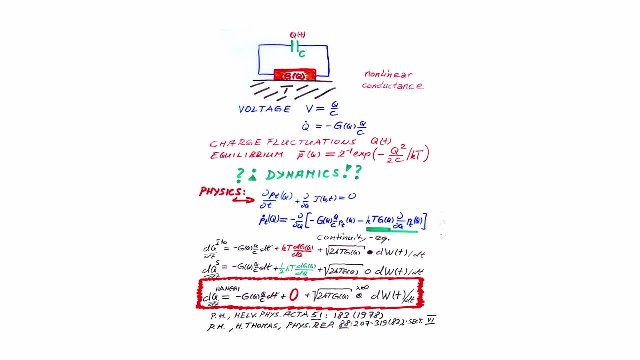 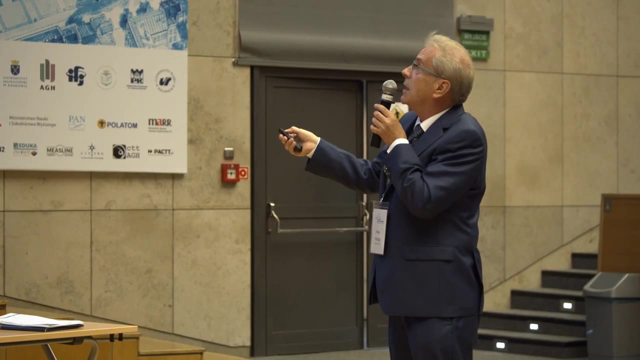 have to take the values at the post-point and not at the pre-point, and not at the midpoint, and when you get here, zero. So you see, with this interpretation you can use the deterministic law and when you use this interpretation and when you have no contradiction, because if you take any, 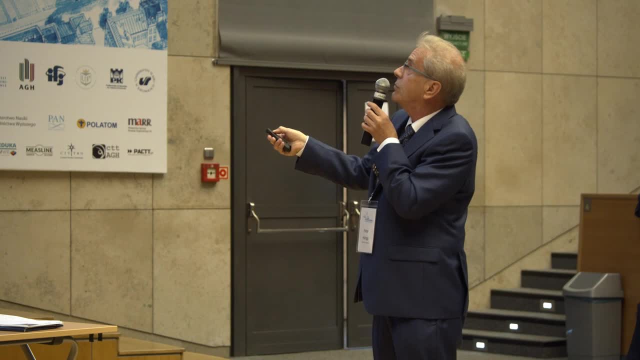 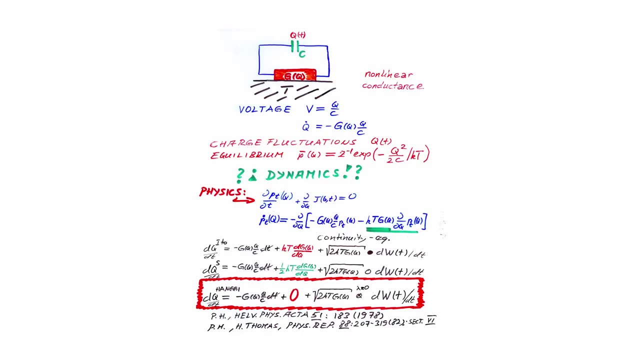 other contradiction like that one. if you would use this here with either Ito's or Donnelly, you would get the finite voltage across the capacitance. That would be terrible, And this is the other thing. and another people thought a long time of embedding quantum mechanics. 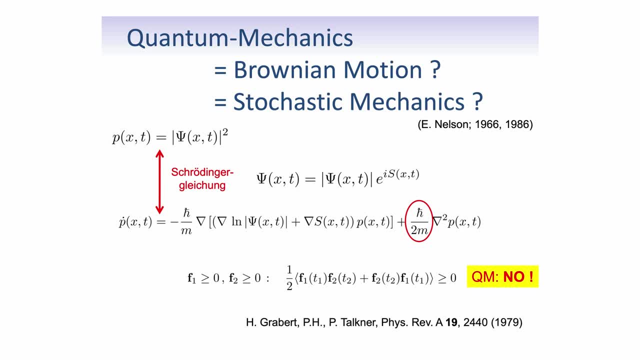 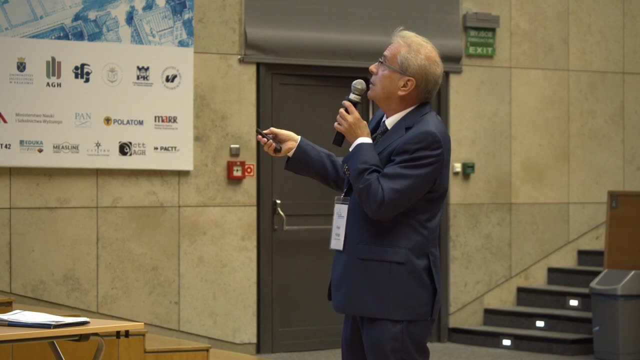 into Brownian motion. That's a little bit the story of abuse. I also worked on this and I showed that with Nelson scheme of stochastic mechanics it's essentially in several aspects not unique. For example, this diffusion coefficient- H by 2, can be chosen arbitrarily and you can 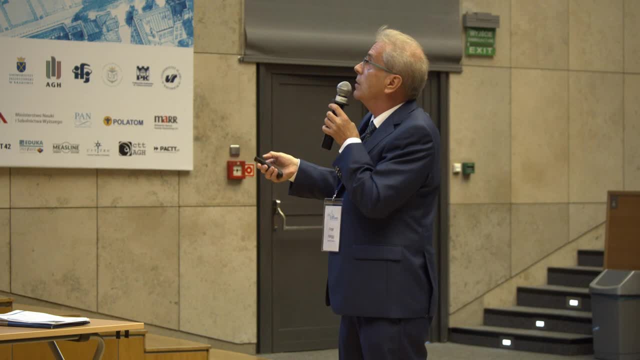 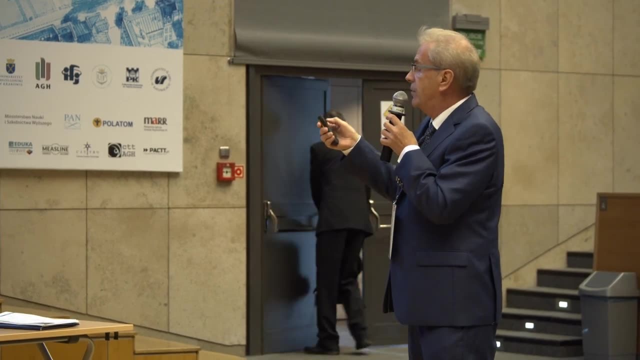 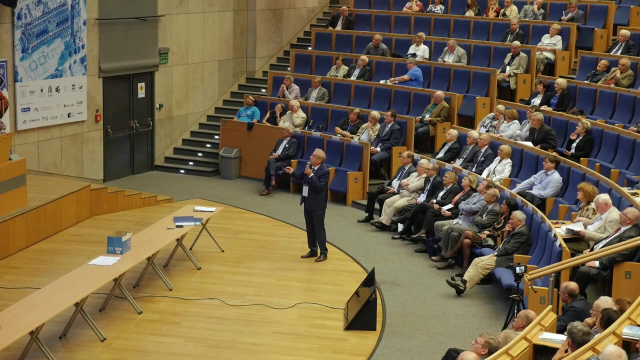 just call. You can correct this part with a constant and, most of all, as you know, if it would ever be a stochastic process you must have in quantum mechanics for positive operators or similarized operators. you would have a positive value for correlation function and 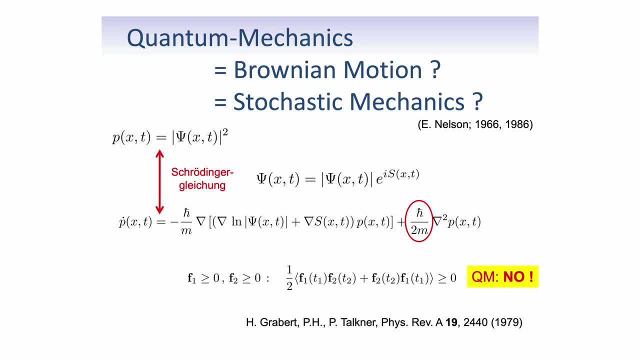 you see here, this is a Hermitian construction of an observer at time t1 and time t2, and in order to get a real number, you take the symmetrization form, And this is: These are positive operators. and then, of course, it's well-known that the quantum correlation. 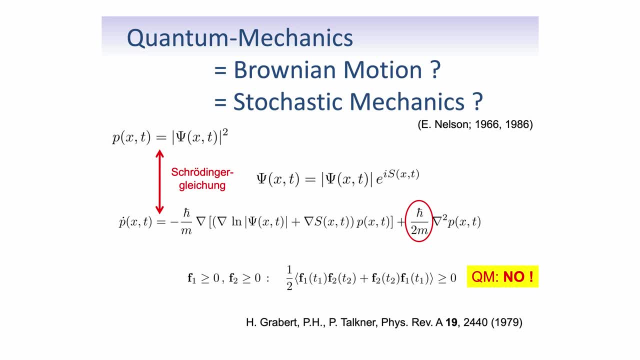 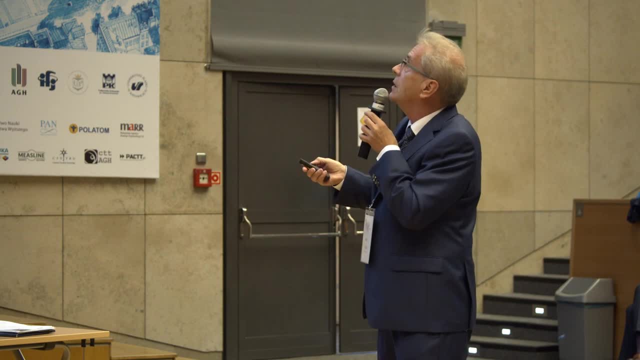 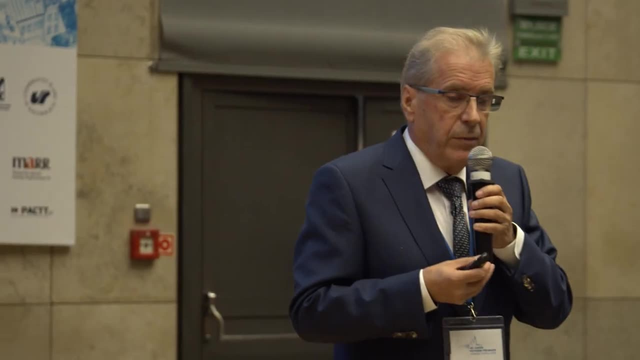 doesn't have to be positive at all. So you can never. Quantum mechanics is never equivalent to any complex stochastic description, Markov or non-Markovian, So it's a no-go. And now I come to a little bit. I have no time to go into detail, but I will give you some aspects where problems still. 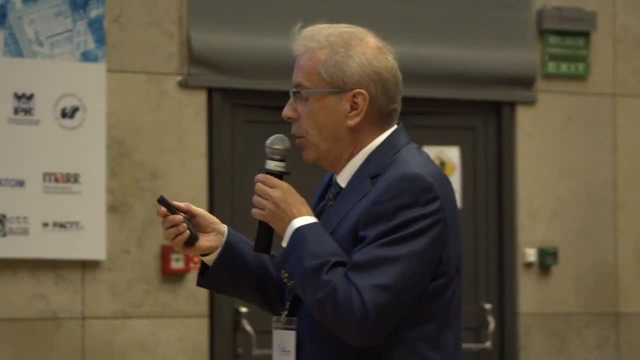 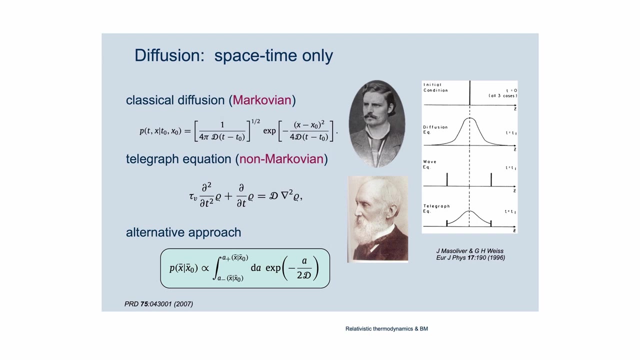 occur in Brownian motion theory. First of all, you are all familiar. You are familiar with Fick's law or even the Fourier law in phonon transport, and usually the propagator is the Gaussian and you start out with a sharp delta function and you see: 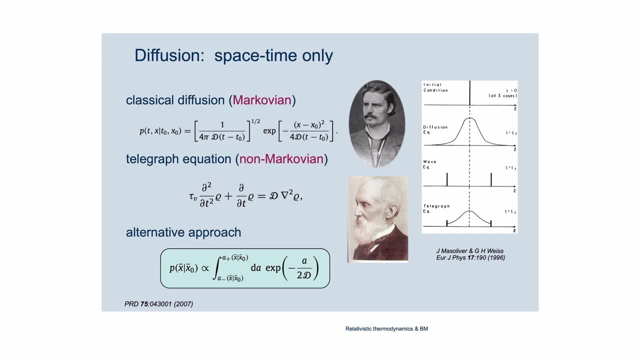 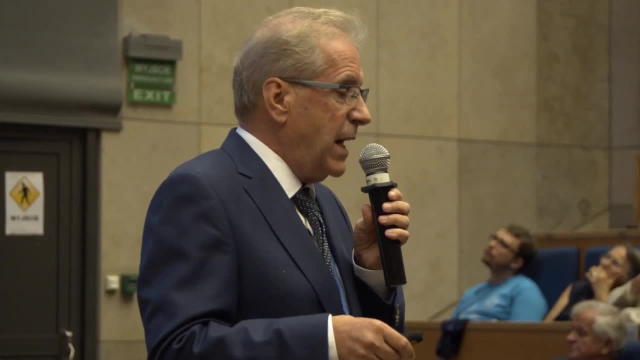 at any later time. t- the support of a Gaussian is on the infinite line. That is contradicting special relativity, but you have, so to speak, a finer probability at any distance away from the origin. That would mean that you have superluminal diffusion, so to speak. 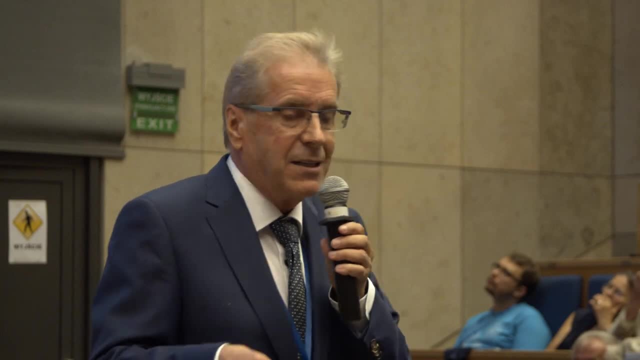 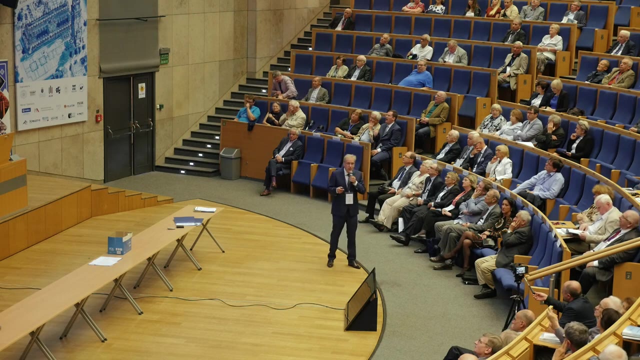 So you have a superluminal diffusion. You have a superluminal diffusion. You have a superluminal diffusion of a finite size particle, which is not possible because it would have to have infinite kinetic energy. Now the question is how to treat, for example, this non-Ecran relaxation, which is consistent. 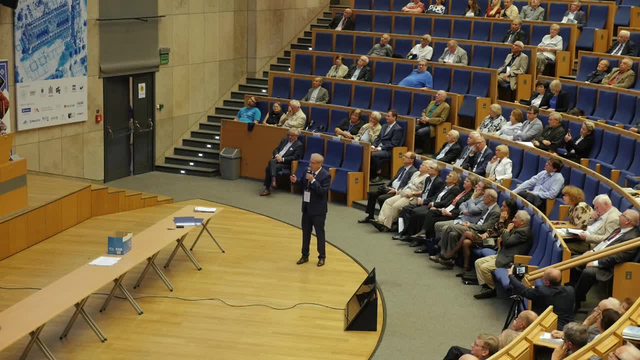 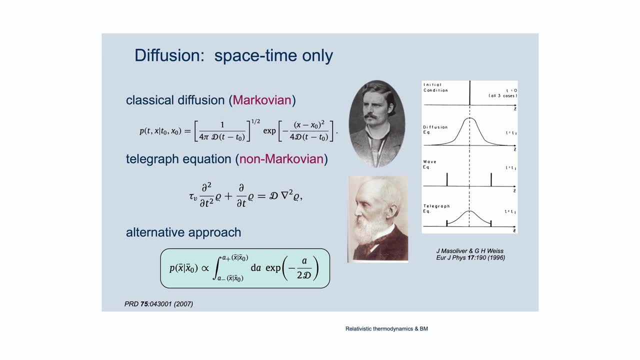 with special relativity. Many people put forward, especially the high-energy community, something like this telegraphic equation here, this telegraphic equation, This telegraphic equation which essentially is not possible, Really possible to get here, no support outside the light cone, but it has fronds. But now fronds. 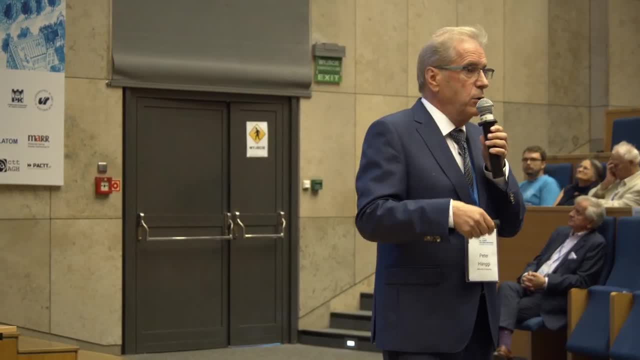 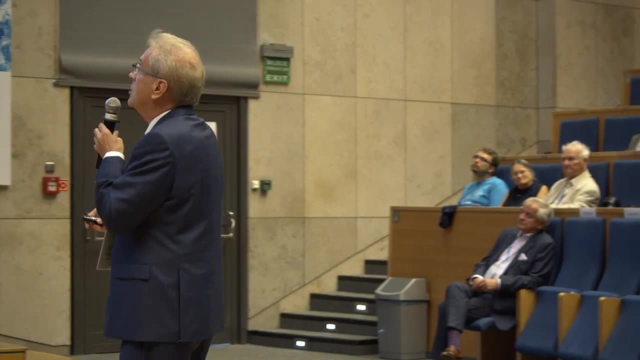 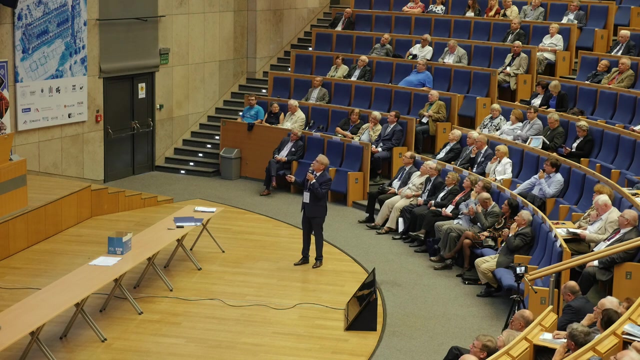 are unphysical For a finite particle to move with the speed of light. it has an infinite energy. It cannot be the correct description, even though it's used in certain high-energy communities, And so we have here a problem. And in addition, with such an equation, it 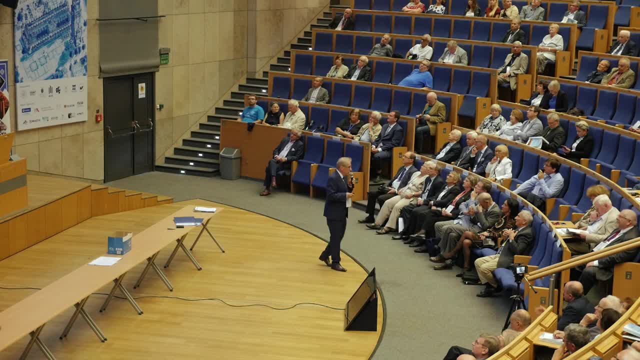 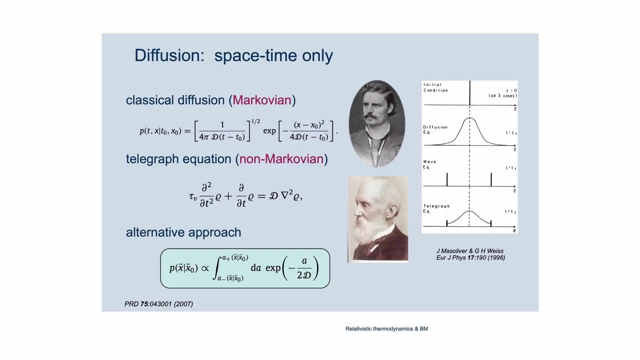 has also been used in phonon transport for the Fourier law. But when you can show you get a contradiction with the second law of thermodynamics. So actually we put forward a path, integral formulation, which I will not explain in detail. But you can actually do stochastic large evacuation, but you have to go from position space into. 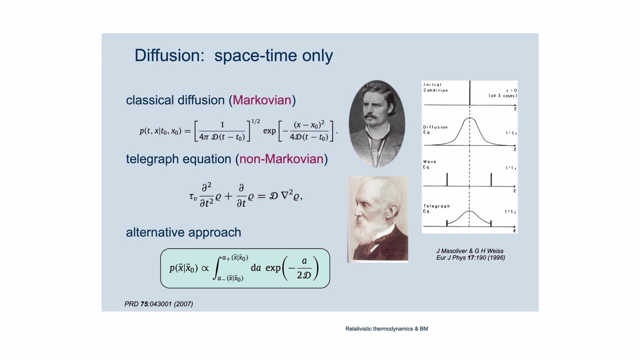 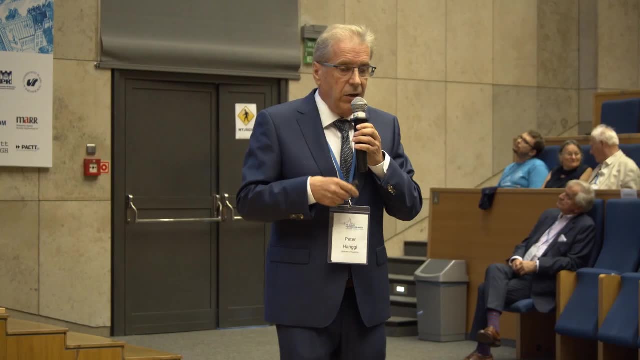 phase space, not into position and velocity, but relativistic momentum. and then you can overcome- And this leads to an old problem of in equilibrium. When you're relaxed, you have a really interesting matter here. It's right, here There's actually a governments. 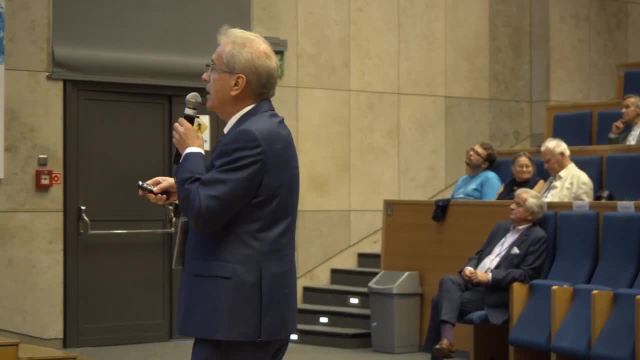 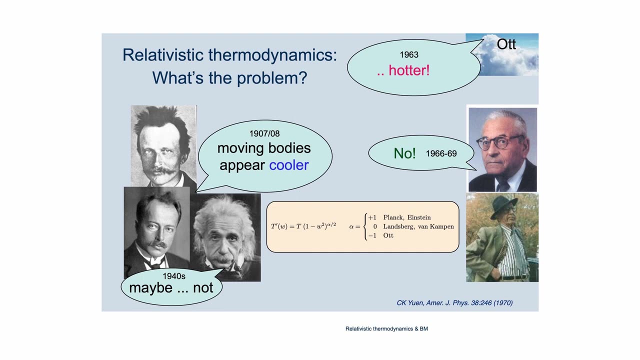 وں situation called the Law of�� of temperature, which says that there's only a MIDI不能 серьile finite that goes from one to ten times the current energy in a mass. SoADCx is an interesting place of death. I express my own opinion of rezid 겠tycul that in this flourishing example of an initial 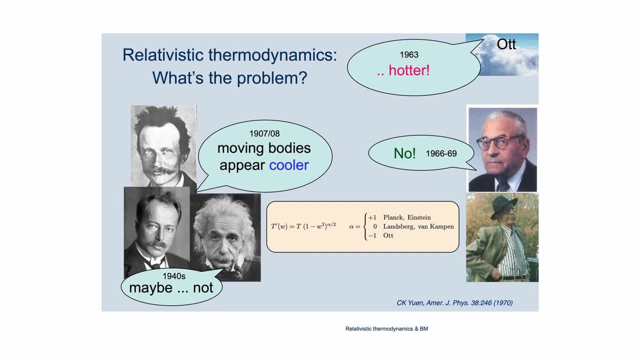 oscillation of sanguine weak states, an initial pulsations. These are generally related to 1963, where the physicist Ott, but also an earlier paper by Sir Etington, claimed: just the other way around, no, it should be hotter. and you see here the transformation law and 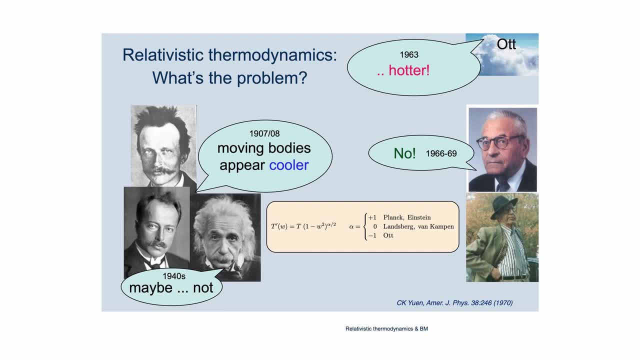 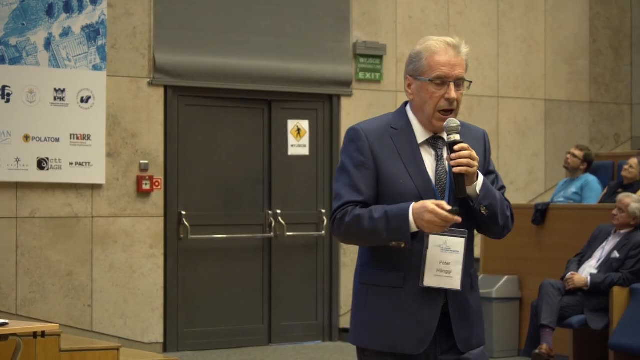 von Kampen was already saying to me once earlier and I met him. this must be nonsense anyhow. and he said the constant should stay, the temperature should not undergo a change, it should stay constant. and an interesting story because Max von Laue worked on this. 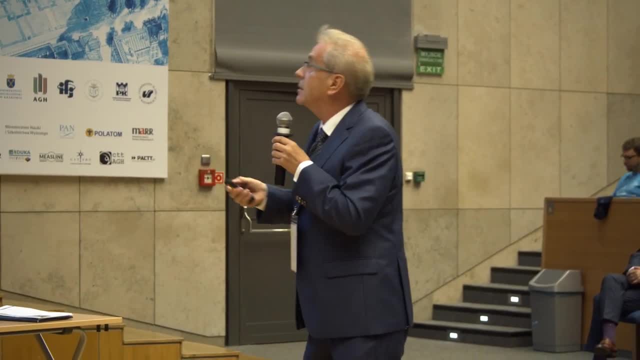 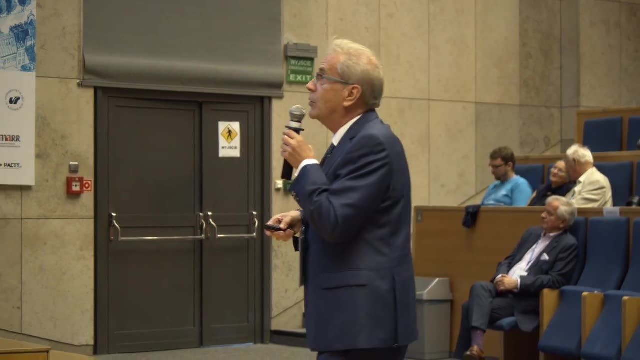 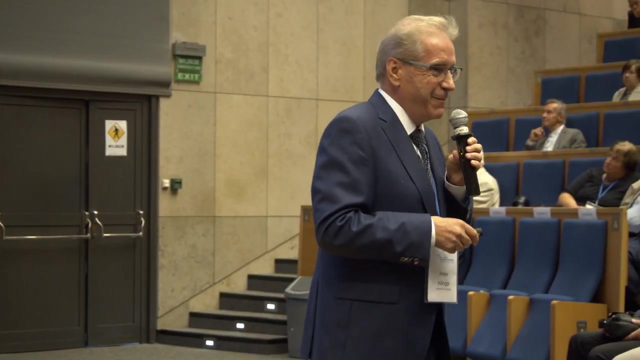 too. and he wrote a letter to Einstein in around the mid-40s and saying that he uses now his result that the temperature becomes cooler. and when Einstein said my dear friend Max, are you crazy? this cannot be right. and when Max wrote back, oh well, I'm a bit surprised. 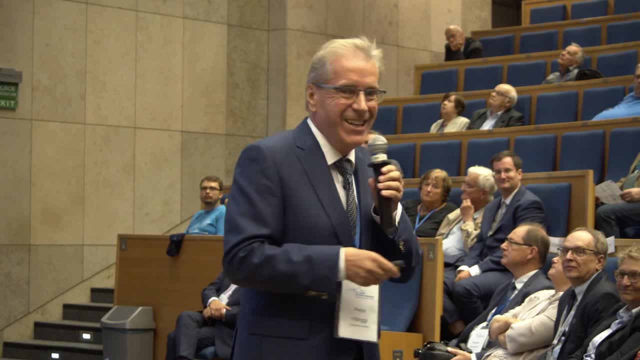 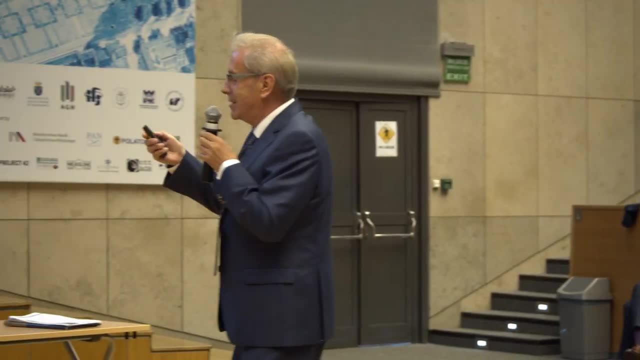 because you say so In 2006,, and I said, wait, I must then be wrong. but he of course didn't have the right answer either, and in the meantime he did, recently, some in one dimension computer. 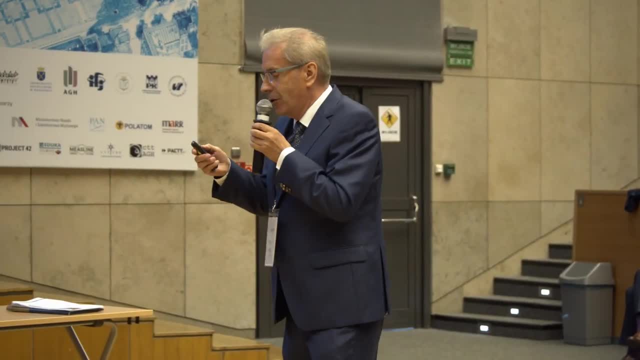 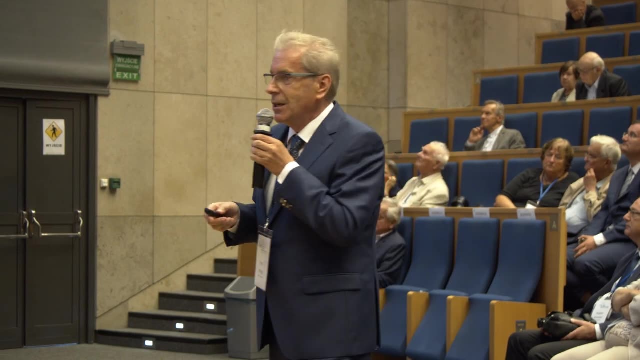 simulation on the binary collisions and we could show- that's a long story- that the temperature that made a lot of headline news in the American Physical Society- that the temperature stays, of course, constant and that does not have a Lorentz transformation. 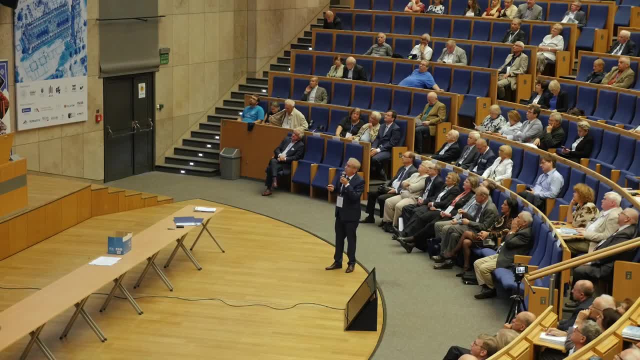 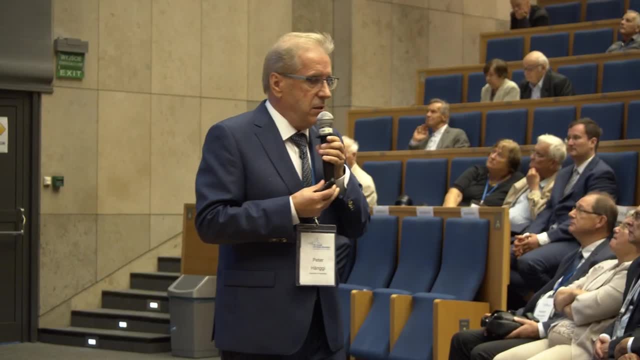 does not obey a Lorentz transformation. That's why we are always saying: what happens when the temperature is too high? What happens when the temperature is too low? So the result of this is, of course, a very interesting theory, and it is also known as: 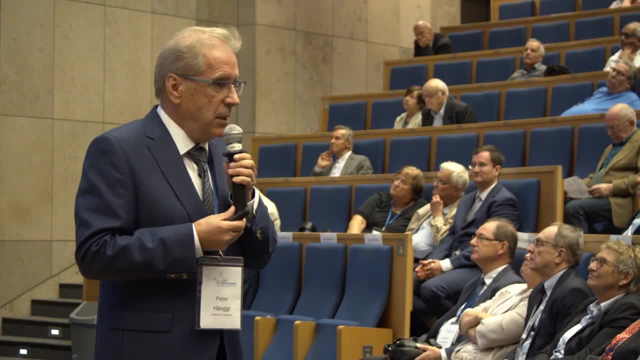 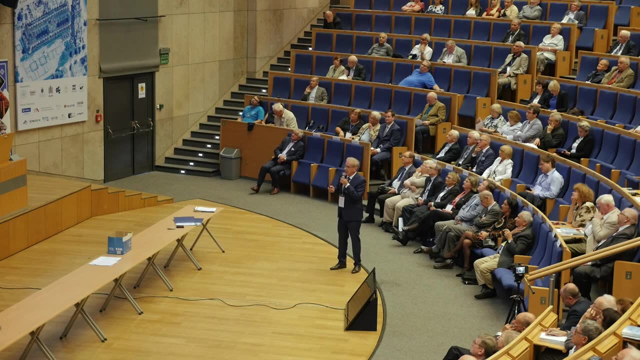 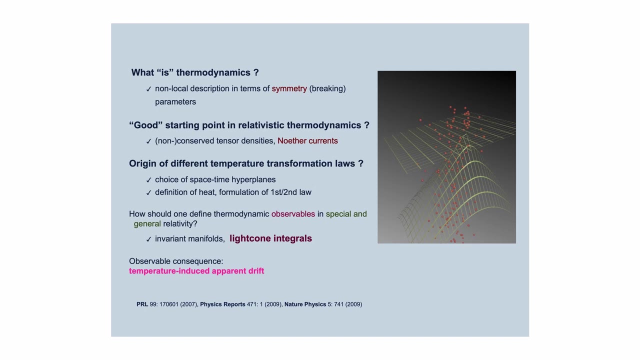 the Fermi-Dynamics theory, which is a very interesting one. The Fermi-Dynamics theory is a very interesting one, So the Fermi-Dynamics theory is a little bit of a new form of information law. Much more important- and this is still an open problem in field theory- is how to actually 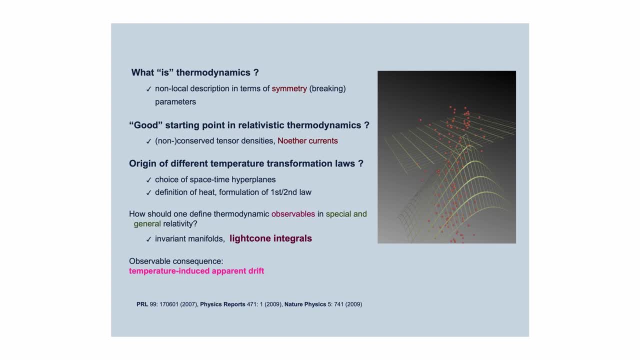 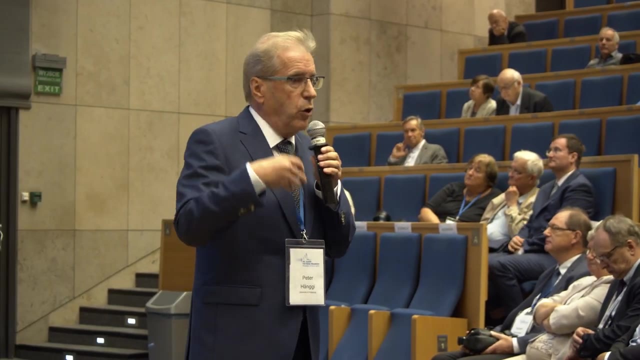 and then that's the first problem. and then, of course, how do you start? because you don't have typically conserved tensor density, see momentum energy tensor for a gas which is confined in a box is does not, does not transform in a Lorentz invariant way from a rest frame into a moving frame. so actually the 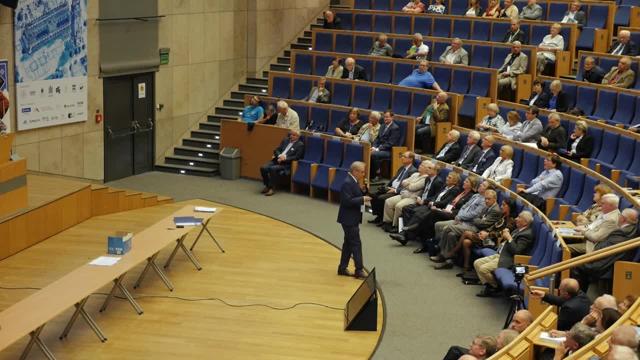 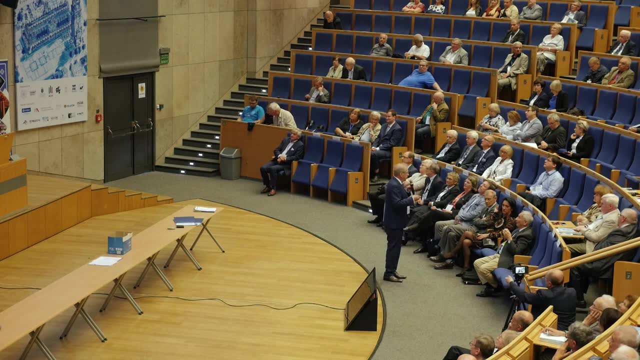 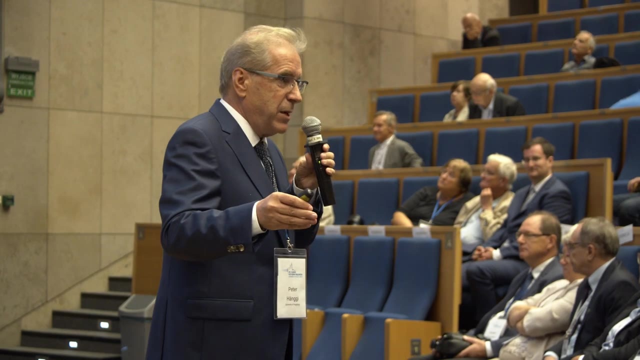 whole problem is that you have to give up isochronicity. and you all have probably heard about the Lorentz contraction, special relativity of length, right, sometimes even being taught. but you will never see, and nobody has ever seen, a Lorentz contraction. you will never see one experimentally done. 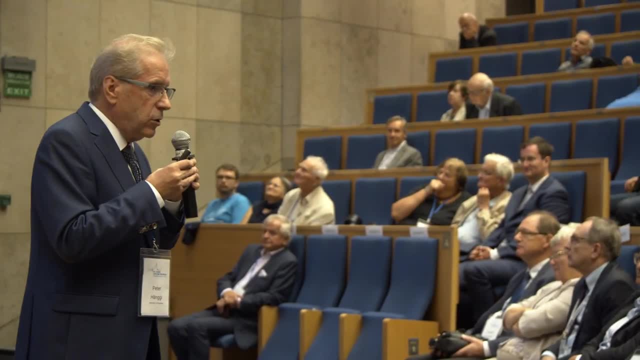 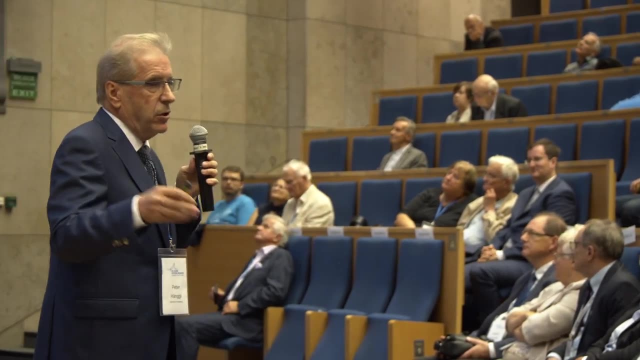 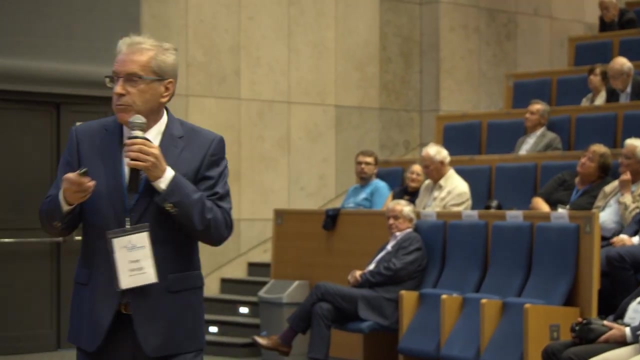 because, in contrast to things which happen at the local point, things which happen isochronous at two different places in space will not be isochronous in in a moving frame. and this is actually the problem: how to define our energy and total momentum? anyhow, we actually put forward to overcome these problems. 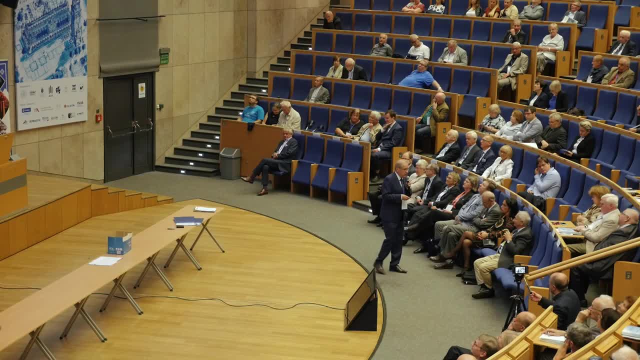 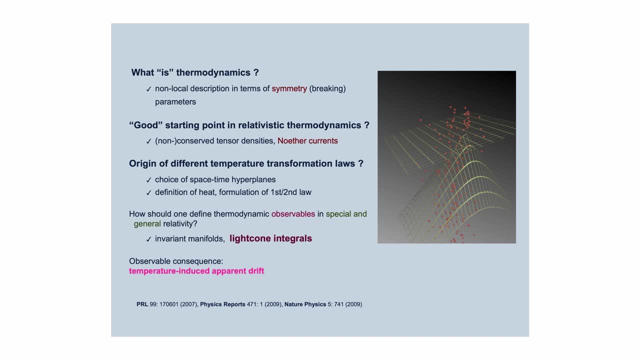 in new insight. in order to have a consistent thermodynamics in special relativity and also in general relativity, you have to give up isochronicity, because all these people try to add momentum over at a constant time, like here at the constant time. we have a hyperplane where all the 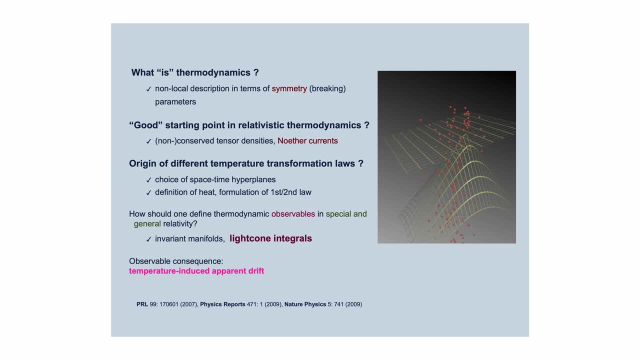 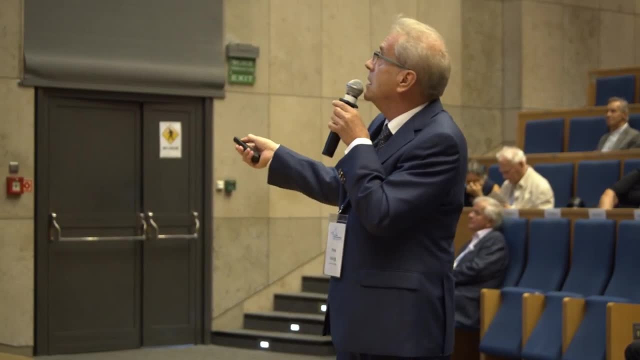 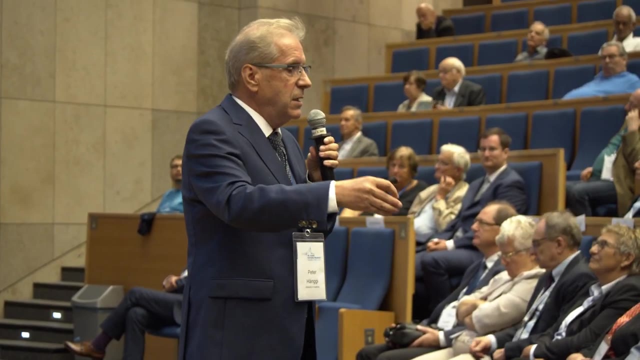 particle momentum would be added up at different places. this will give contradictions and of course we say basically the theory in our nature physics work here is that one has to go back to light cones, because this is a big problem. distant stars from different distances need different times to go to a certain. 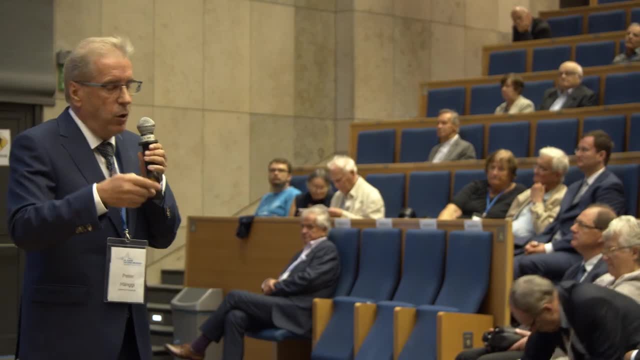 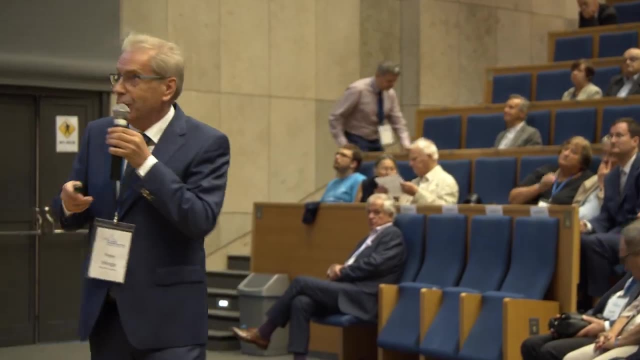 photographic plate and all this has to be built in. it's too complicated to be two weeks to talk about it, but I'm very proud of this photographic thermodynamics which is finally solving this problem of thermodynamics, at least in special relativity. I have not gone yet, but I hope to come back to this topic in the next part. 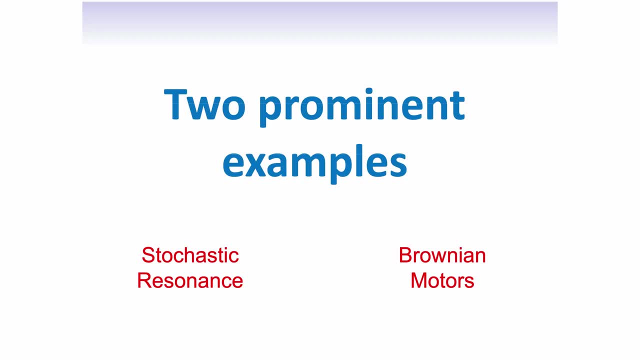 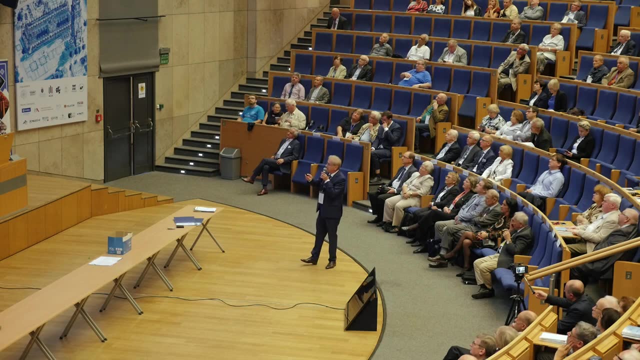 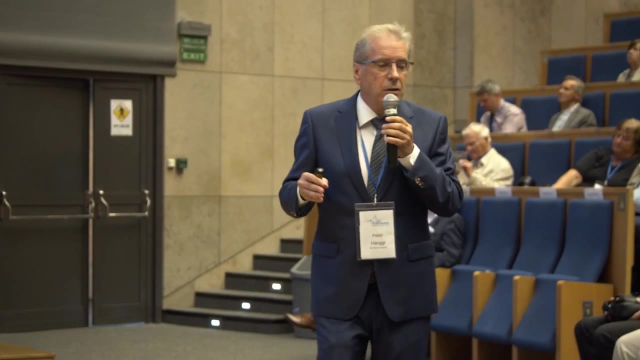 to general relativity. Now I'll give you two examples of Brownian motion-induced useful effects for mankind. One is stochastic resonance And essentially, in a nutshell, it is the following: You have a very weak signal. My wife talks very softly and wants to tell me something. 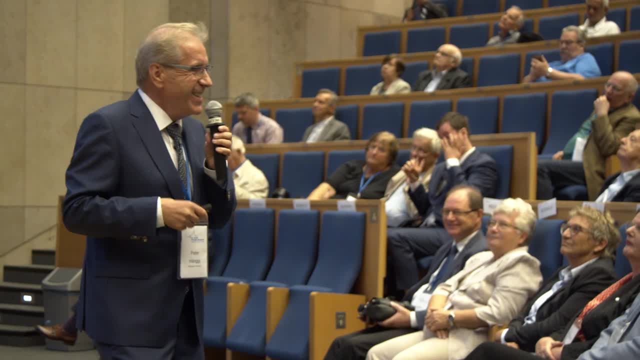 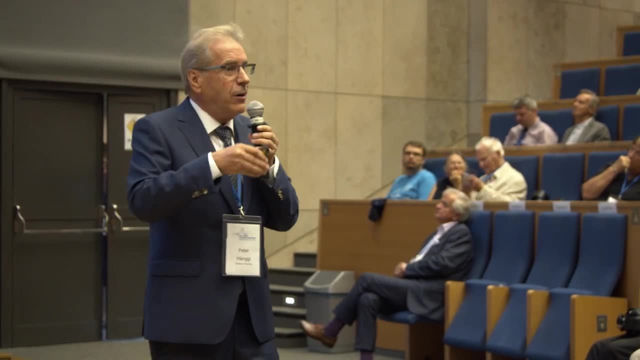 I say what did you say? Of course she says I have a hearing problem And how could I actually do something to get actually over that is, namely in presence of noise, if we are actually in the party in presence of noise, sometimes you feel that 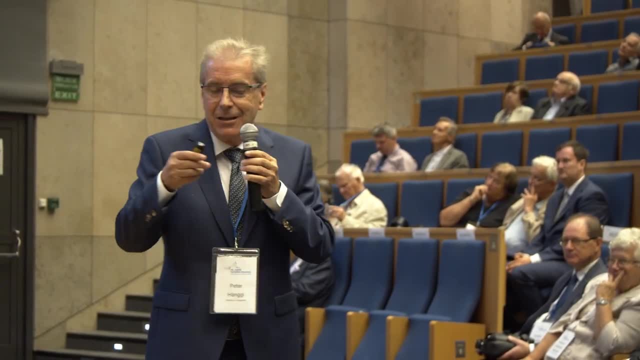 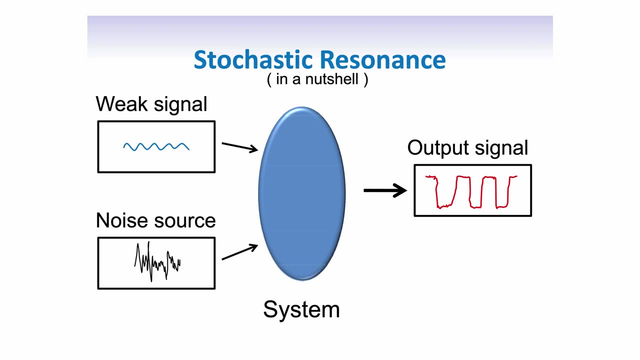 you understand better what somebody is saying in the silent voice. So you have an amplification, You have a weak signal And you have presence of noise. And when you have a non-ear system, if a threshold system- and this is the effect of stochastic resonance under 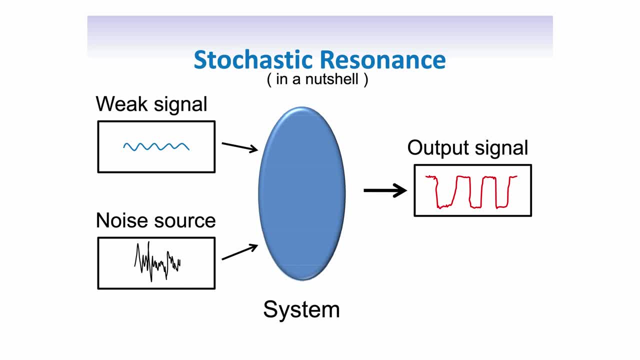 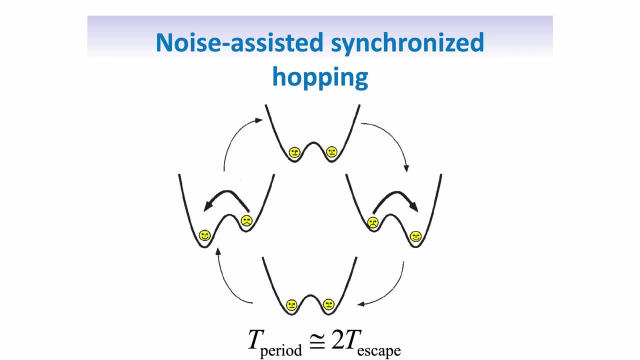 certain conditions- not always under certain conditions- you get actually an output signal which is amplified, Which is amplified OK, And essentially this is that you get a noise-assisted synchronized hopping between. this is a model for this effect where you have a bistable potential. 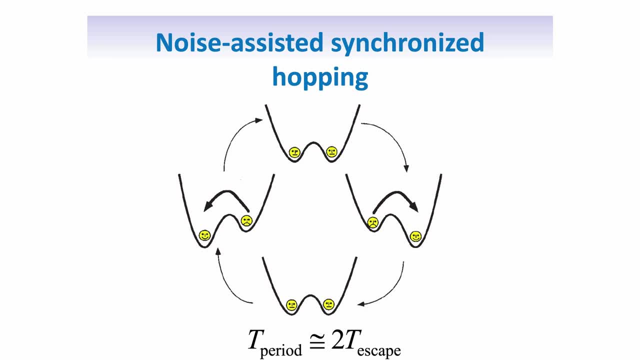 And you tilt it to the left, And you tilt it to the right. So you have two times an escape. Here you take advantage of this barrier is lower. Here you take advantage of the barrier is lower. So over the full cycle you have two time points at half. 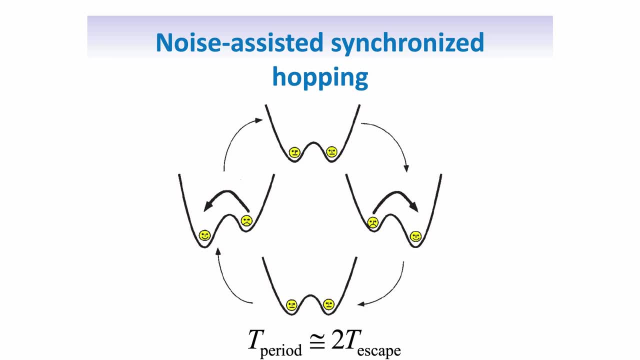 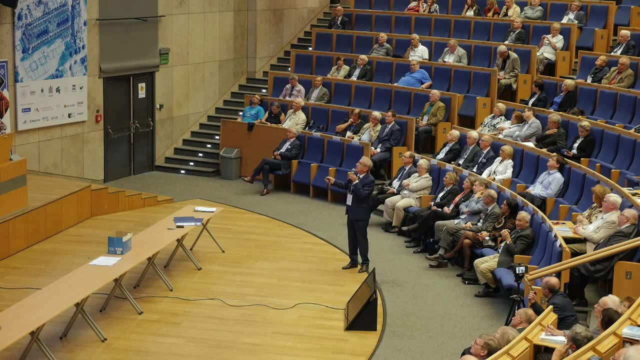 period where you have an advantage, Where you have an advantage to hop. So we have here essentially a synchronization between a deterministic driving period where we tilt the bistable potential, like that, And the random timescales mean value of the escape time, And you can do, you see, this even in simulation. 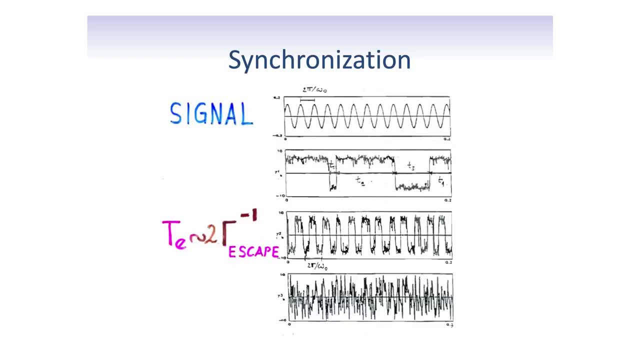 You have a signal And in absence of a signal, you have random hopping, And under the right dose of noise, if the dose of noise is appropriately right. you see, here you get some something like a stochastic synchronization phenomena. Too much noise is bad. 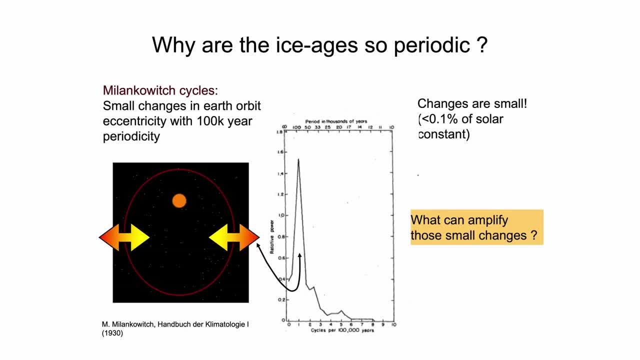 Too little noise is bad, And this is how the whole field started, Because people had three points of the ice ages And Giorgio Parisi and other people made a diagram, calculated the power spectrum And they found a peak of 100,000 years. 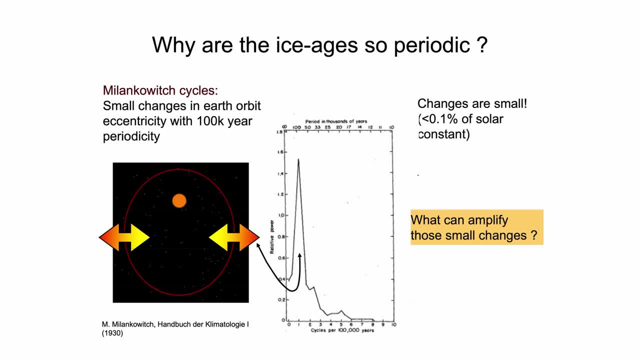 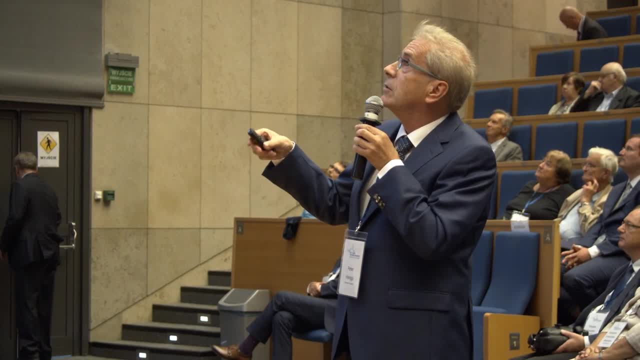 And one knows that the giant ice ages are displaced by about 100,000.. And we think there is of course all this astronomical noise about and also earth noise, And the Milankovitch cycle has a timescale of the sun, of. 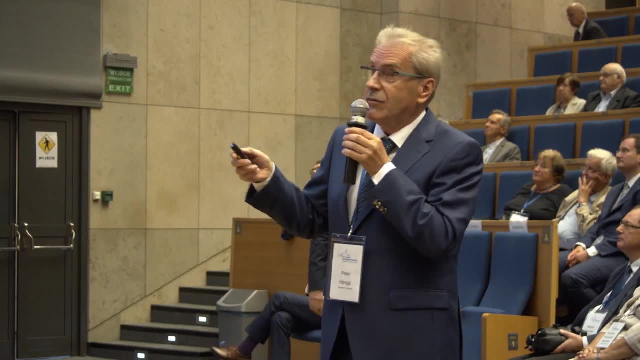 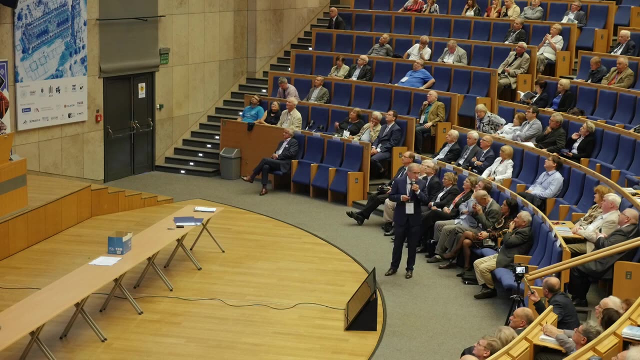 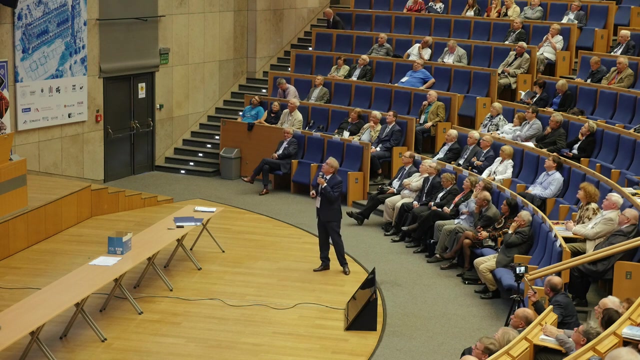 about 100,000 years, But nowadays we don't have evidence that this is the correct explanation, because you have only three points. However, now talking about climate, which is now important, everybody talks about what's happening with the climate. there is occurrence of ice ages on the 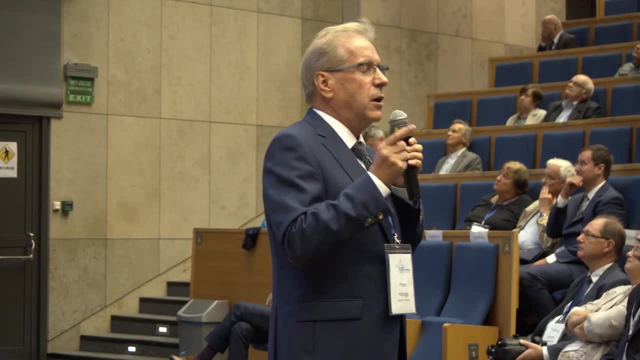 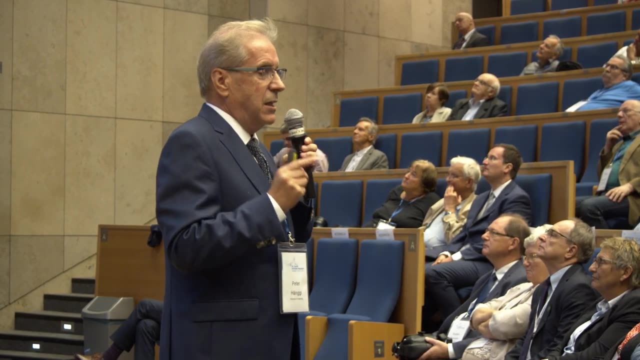 smaller timescale, namely of so-called Dansker-Höscher events, which have a periodic timescale of 1,470 years. So you're off in 1,500 years And we have here data of many years over 100,000, 200,000. years from the Greenland Ice Sheet Project. And now the question is: why do we have more small ice ages occurring on a timescale of 1,470?? And this is actually based on the climate model, The climate model which goes back to Rumsdorff and other. 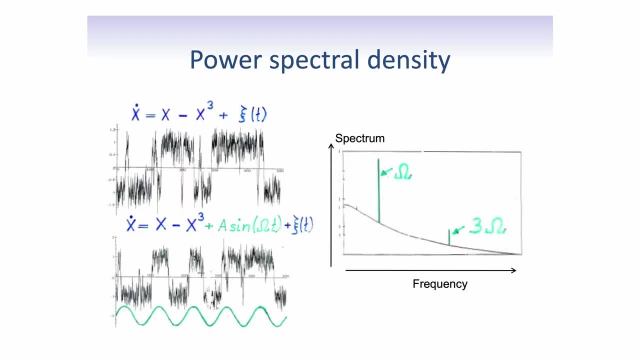 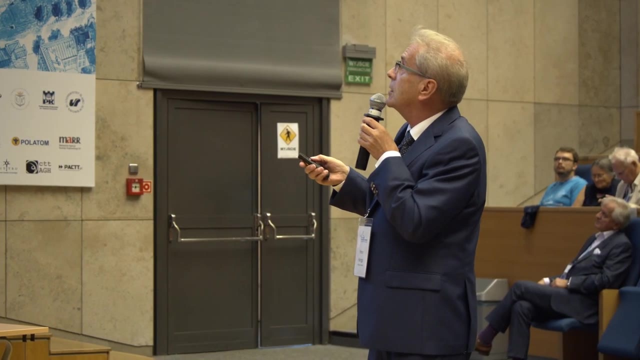 ones where actually stochastic resonance is at work, without going into more detail, And essentially, another important thing is that this deterministically driven stochastic system has a total different power spectrum. The Wiener-Kirchner theorem must be generalized to this temporary driven systems using Flocke theory. 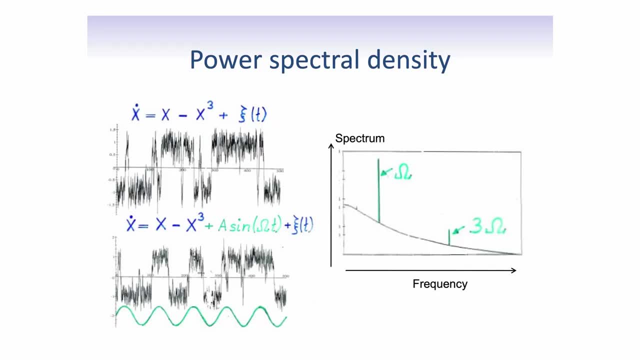 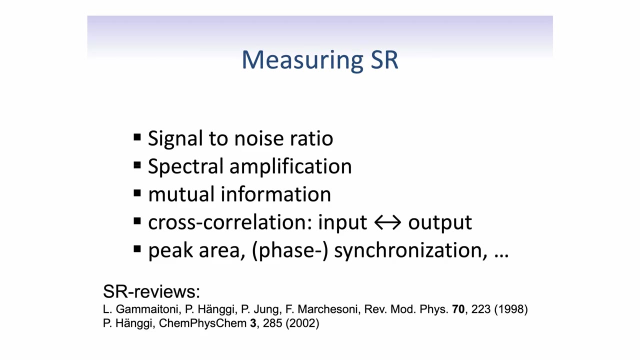 And you see that you will never get in a somatic system a response at 2 ohms, Only at 1 omega, 3, omega. So this has led to patterns to really distinguish between exact symmetry and not exact symmetry. Nowadays we have all kinds of measures. 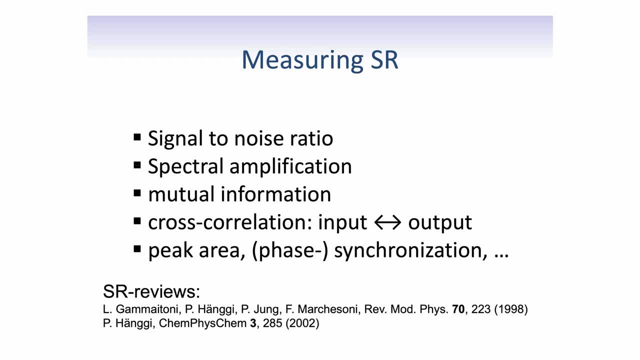 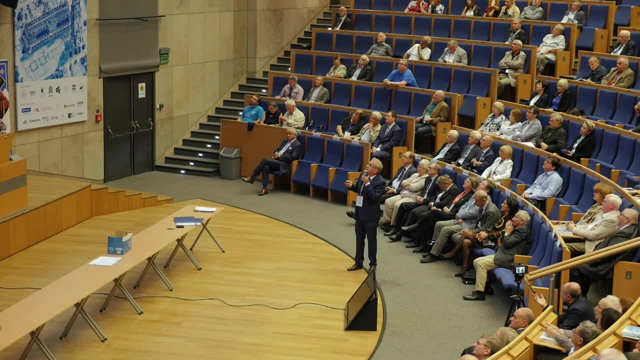 We don't need periodic signals, We have also arbitrary signals. We use information measures like trans-information, And here we have two reviews on this effect. And now I give you a summary of this effect. what an amplification takes place for a certain amount. 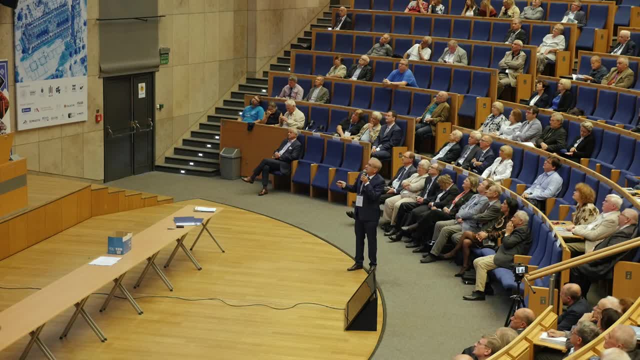 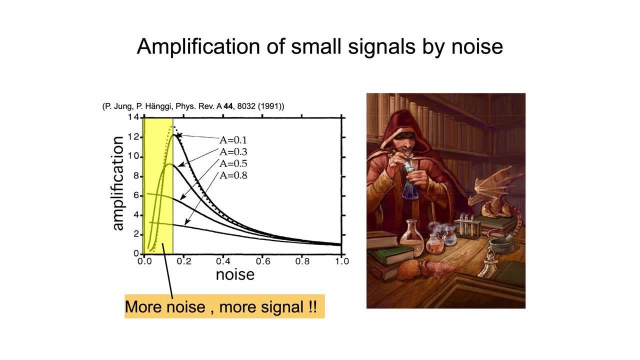 of dose here, a maximum. If too much noise is bad, too little noise is bad, And then in this region you get more amplification. But what is more important than the maximum is the slope here, because that is the gain of amplification, if you look. 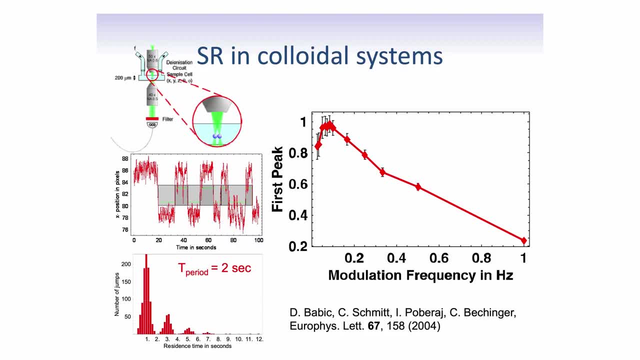 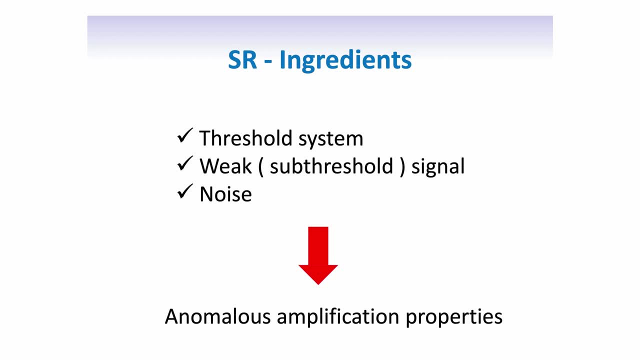 at the slope And, as a matter of fact, this has several. I will skip that one. Nowadays we have an important effect because all you need is some kind of threshold system Doesn't have to be a barrier, It can be just a threshold, a neural. 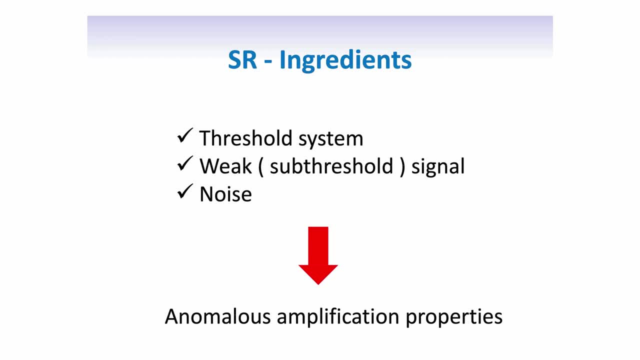 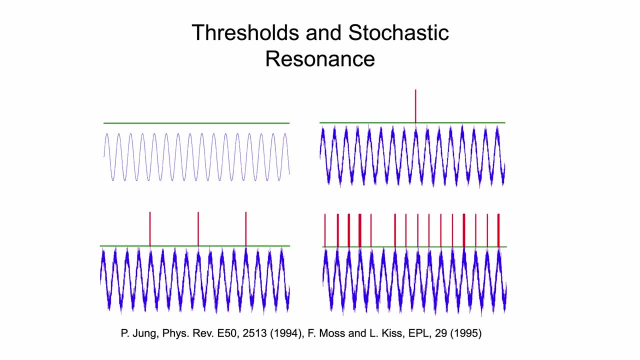 threshold. You need to have a weak information type signal and noise usually is ambient around for free And when you get animal amplification properties- and this is essentially here- if you have a threshold, for example in hearing, you don't have enough spike in your 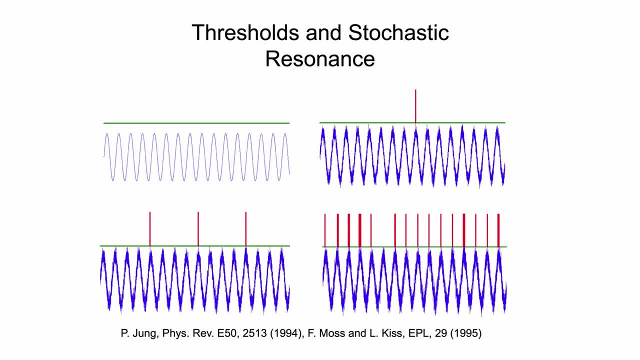 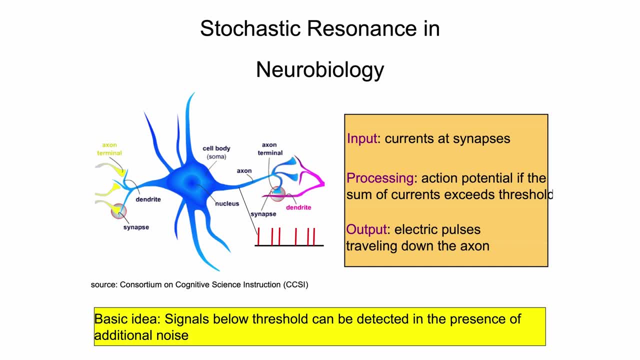 hippocampus, you will not hear what you say. But if you have a little bit of noise, when you get more spikes and the spikes are being transformed in your hippocampus to dissolve the information, And this, of course, is taken place in 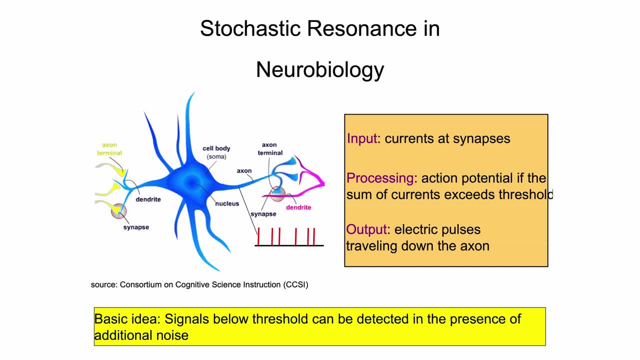 the nicest example why this becomes now so famous in neurobiology. We have such threshold systems all around And you can read: we have input currents, a synapses processing along C axons and then goes into the hippocampus And then you can see and hear and speak things. 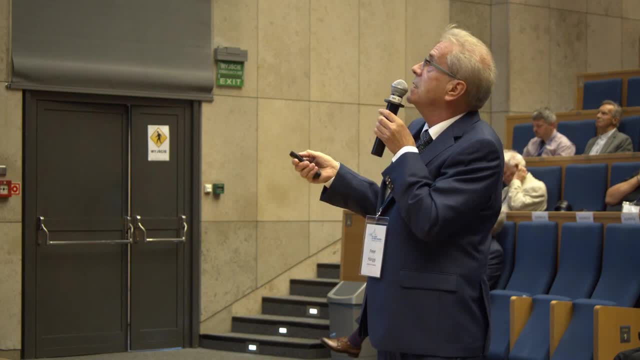 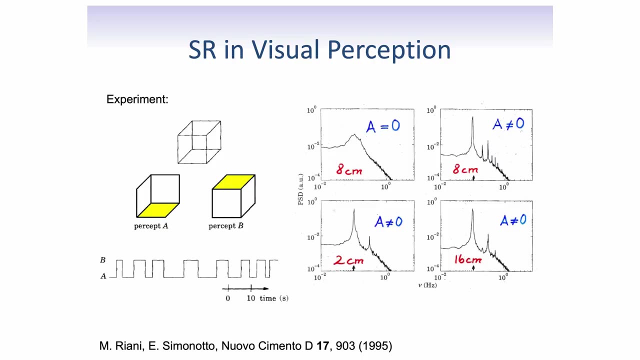 And one important, just one important little example is this: where you can see this, You have here a cube which is visual perfection. Now you can see this cube under this condition until you focus on the base floor here or you focus on the top floor here, you see two different you. 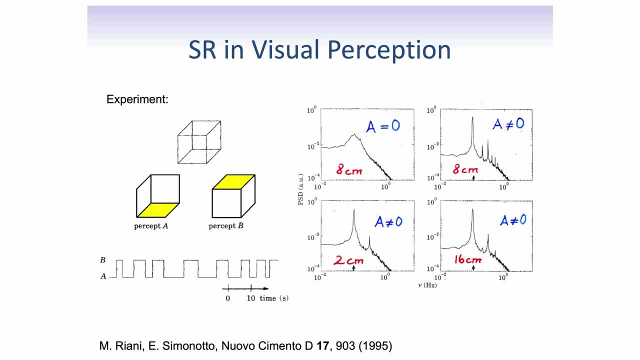 should see two different percepts of this cube. Now people did experiments where you can actually move this point from here to here in a certain frequency and you see that in absence of this perturbation, that the power spectrum of those clicks of the response changes a lot. 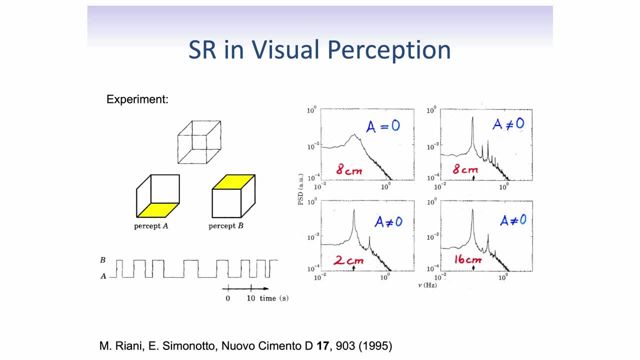 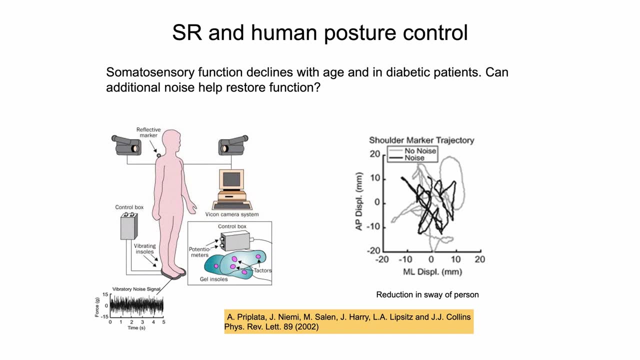 And here you can actually relate that to stochastic resonance, let's say, Nowadays this is the whole industry, Namely it's called stochastic resonance therapy. You find it in all kinds of doctors' labs or also in what is called in the chiropractic labs or physiotherapy labs. 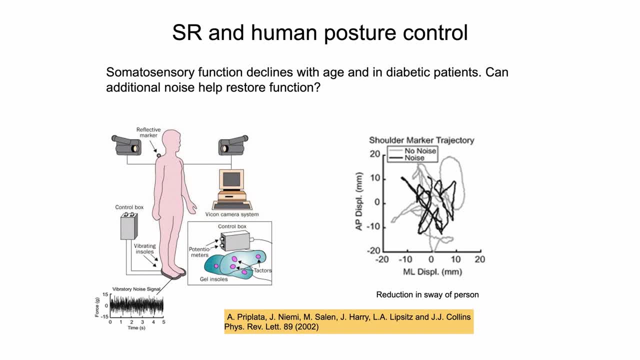 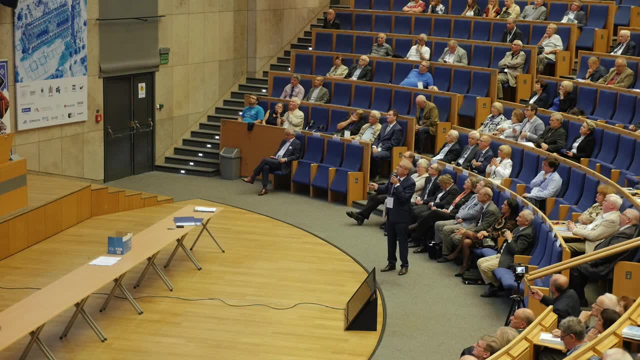 I mean all sports people usually go before they go to the Olympic games and such. For example, moving vibrating plates: Here is actually a beautiful experiment where you have young man and older man standing on a platform which is vibrating with mechanical noise. 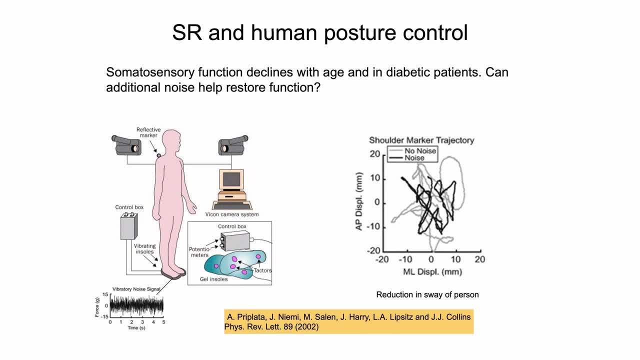 First of all, you adjust its sub-threshold so the guy doesn't feel anything. You reduce the vibrations. he doesn't feel anything, And when you measure the sway, everybody has a little bit of shake and he cannot stand totally still. 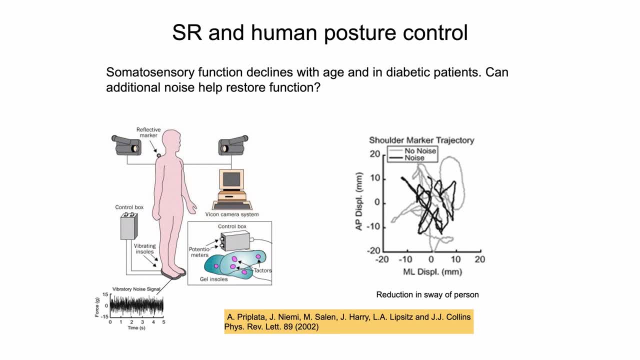 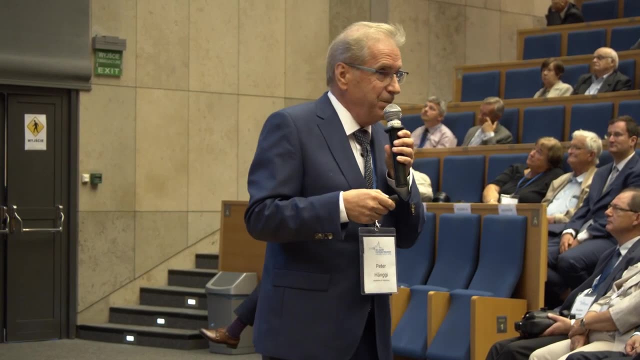 And of course in older people you have more sway than in younger people. right And now they add noise and they find out that actually the stability of older people in walking improves to a certain measure, which is typical for young people. 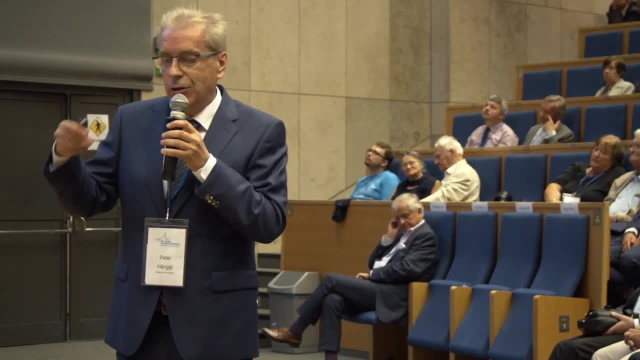 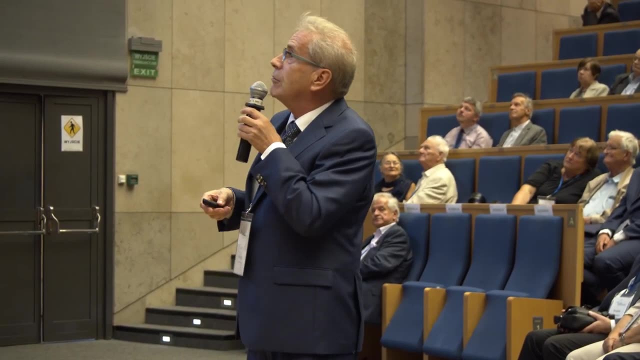 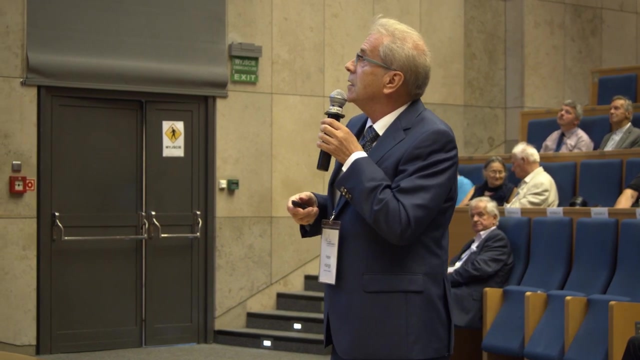 Can you imagine actually you stand on these vibrating plates and when your motor control is much better? So actually there is something here around where actually giving the right dose of noise will improve, so to speak, the impairments of age-related stability, motor control. 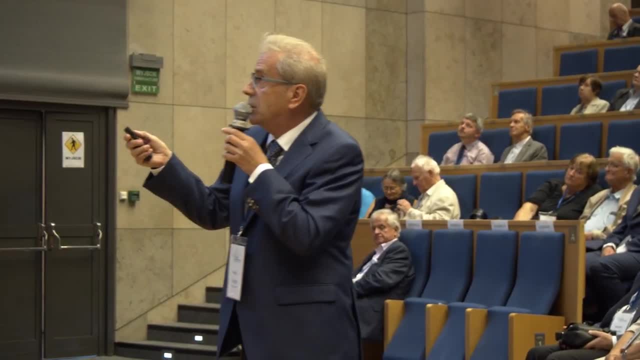 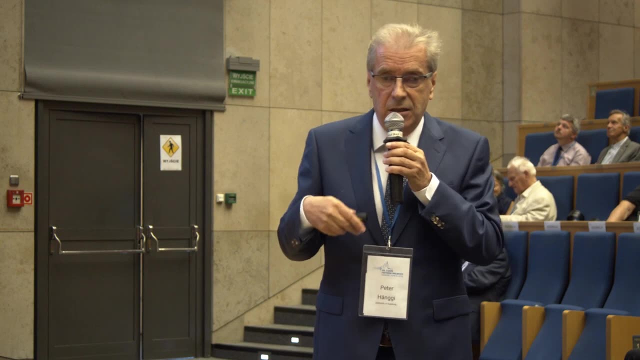 This is actually very useful. Nowadays we have also magic socks And, as I say, these plates are actually working all over. I had a student of mine which took one of the antibiotics and he could not stand anymore, could not really walk and could. 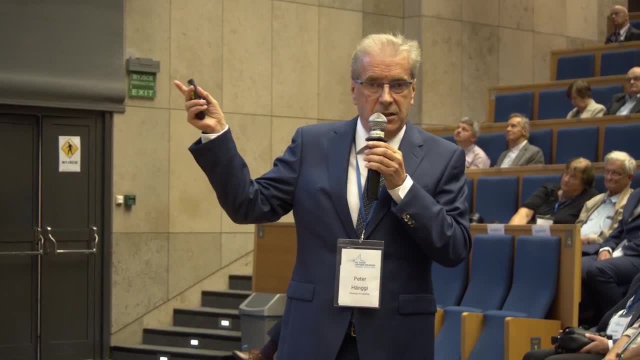 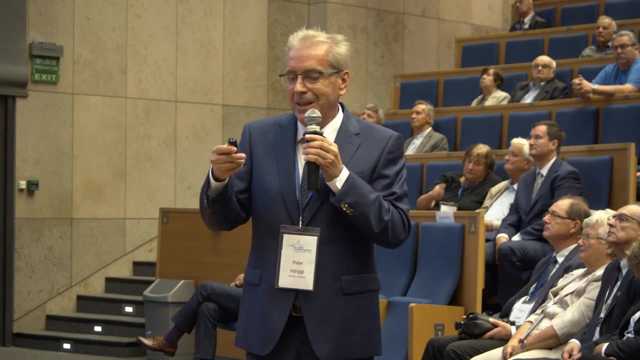 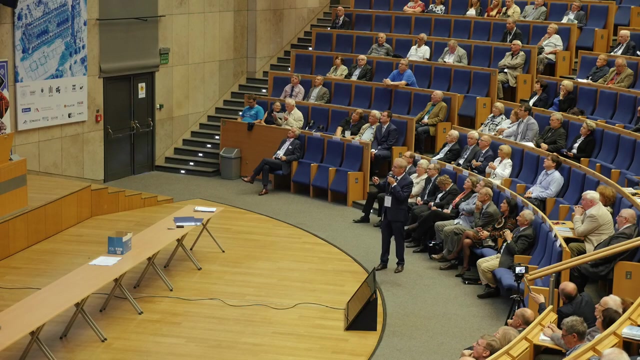 not even drive bicycles. After two years standing on such plates, he came back and he walks now. So it's stochastic resonance from our physics. people have an immediate effect over a time scale of 20 years, And here you see such older ladies standing on this plate. 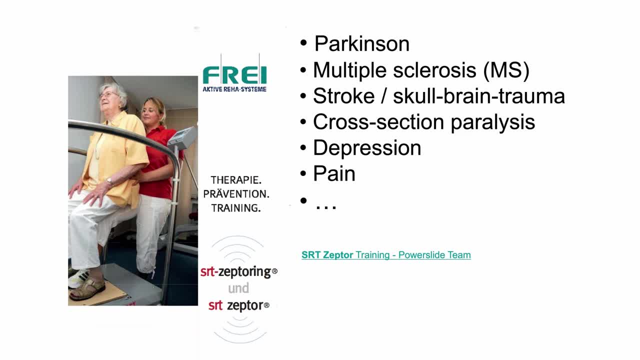 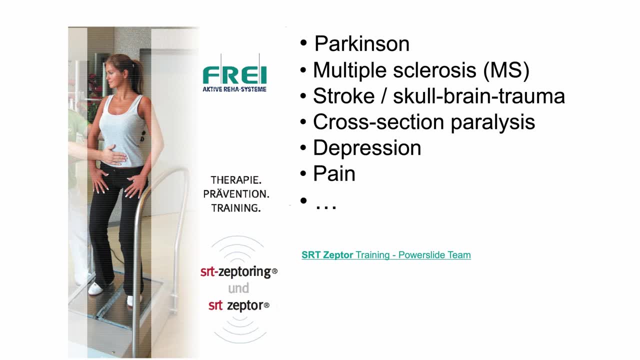 which are typically shaking around, have a hard time walking, and now, if you stand, you have this effect. Of course, this is not real, but it goes in that direction And nowadays what is important, that we also for doctors. so 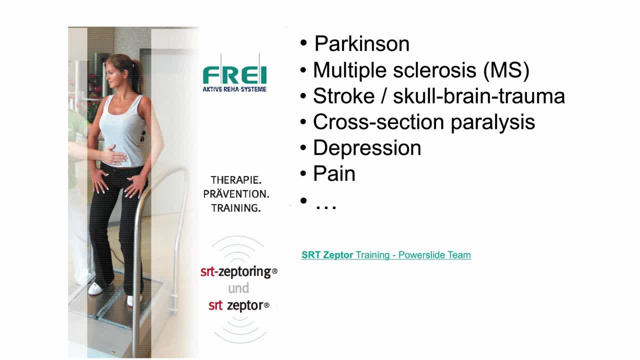 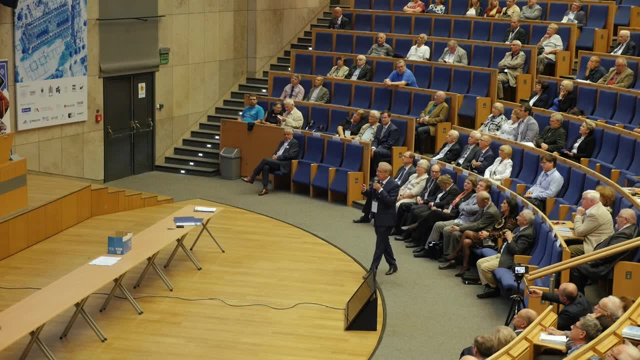 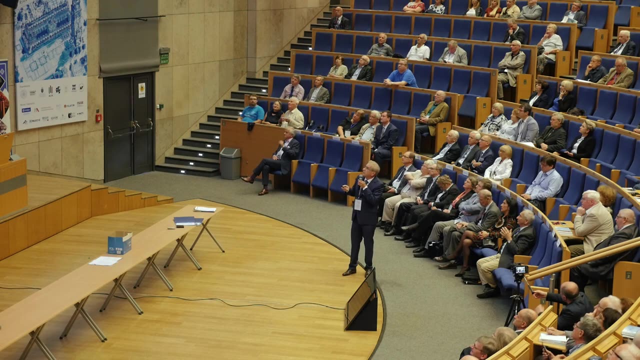 brain surgeons have special gloves which actually are vibrating either with mechanical noise or also works with electrical noise, In order to really hand the operation with most precision. OK, so nowadays we have also a phenomenon: quantum stochastic resonance. I just have enough energy physics paper on this, but I 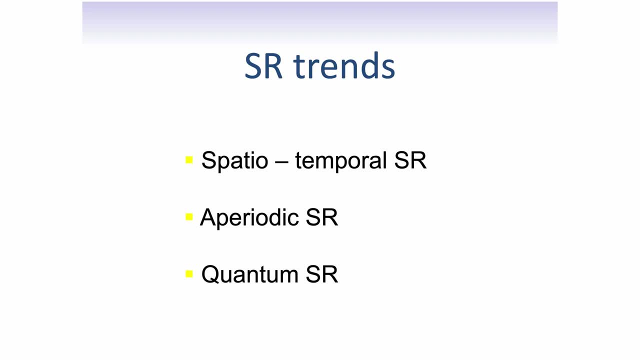 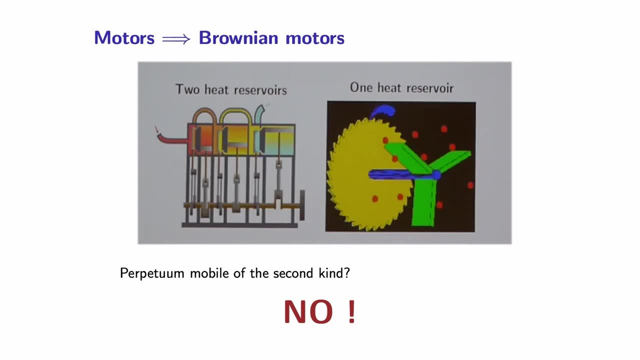 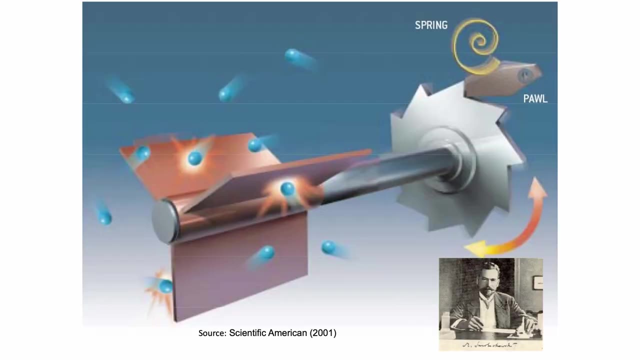 will not go into this field which is presently active in the quantum stochastic, in the quantum regime. Now I go to see more to something which has brought up by Mr Smoluchowski, Marian von Smoluchowski. This is a picture from the Feynman Lecture, so to speak. 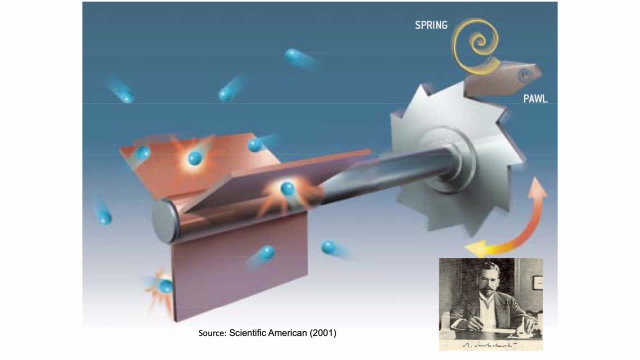 where you have a ratchet and the pole and the vane and you can see that if the molecules hit from the right side, you can turn and the other way around is more blocked. This is actually in the books of the Feynman Lectures, but 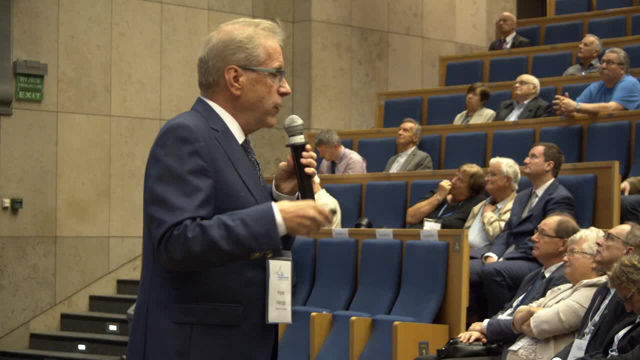 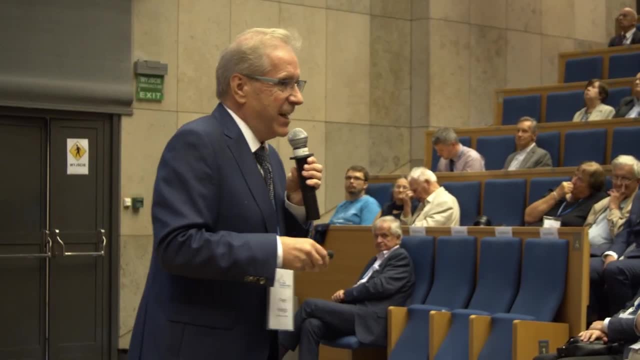 nowhere do you see Smoluchowski, But I know from reading the Feynman stories that he was reading the Göttinger Lectures of Smoluchowski of 1913, and Smoluchowski of 1915.. Smoluchowski has written precisely this stuff since. 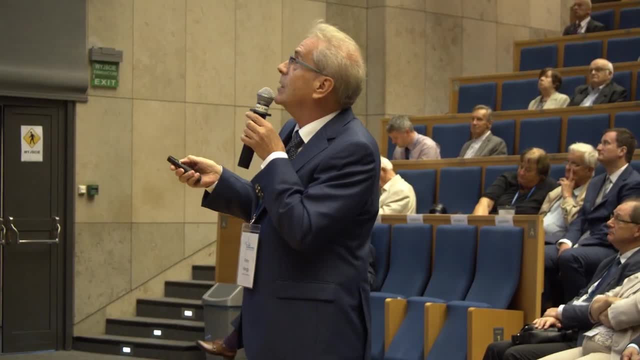 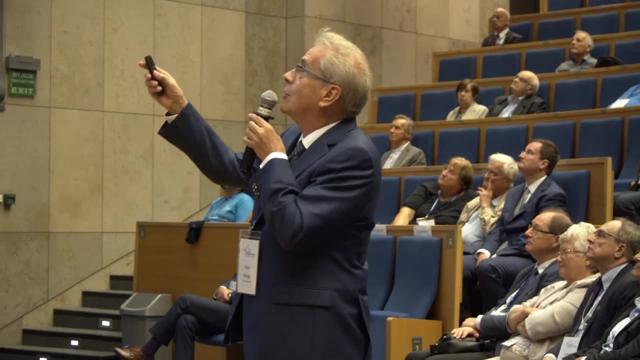 Smoluchowski's ratchet is part of his Göttinger Lectures And even here earlier at the physical society meeting in Germany he actually talks about in German, about Zahnrad means ratchet and Sperrklinke means pole. 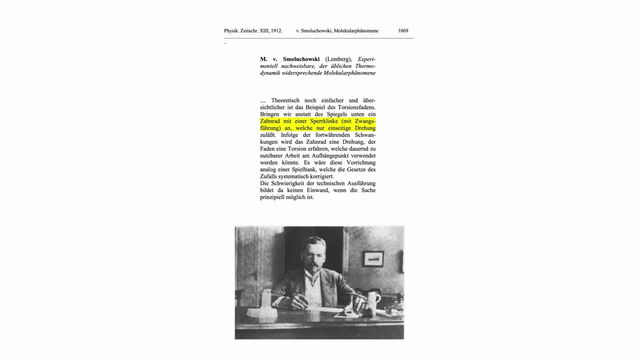 And he describes that, what he says, that you cannot drill a hole, it will not work, it will not be a system. but you cannot have a Maxwell-Thame one. And it's so interesting actually that the masters of that meeting in 1912 asked all kinds of tough questions after. 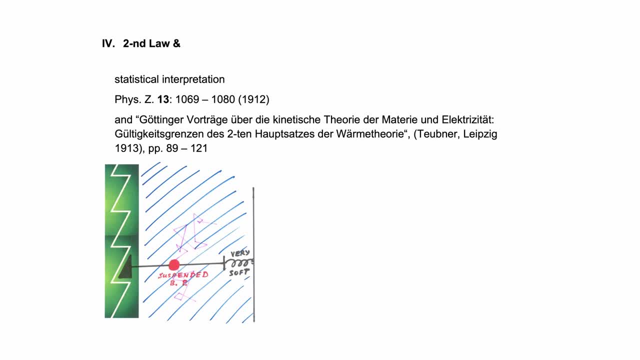 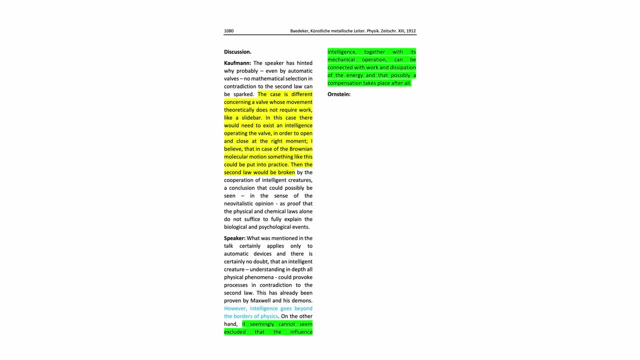 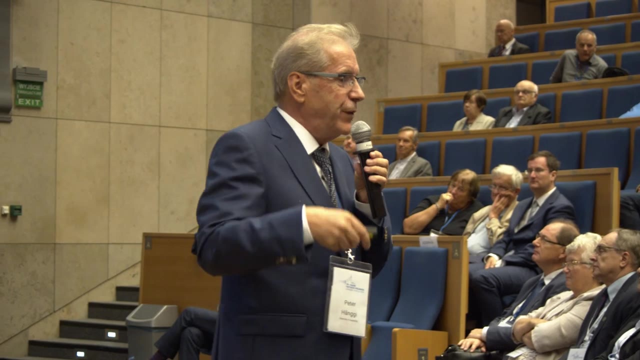 his talk. This is actually the description of 2013.. And I translated that into English and people asked him: is it not possible to use somehow the Maxwell-Thame one and if you would have enough intelligence openings and so on and no friction, to actually make a perpetuum mobile which? 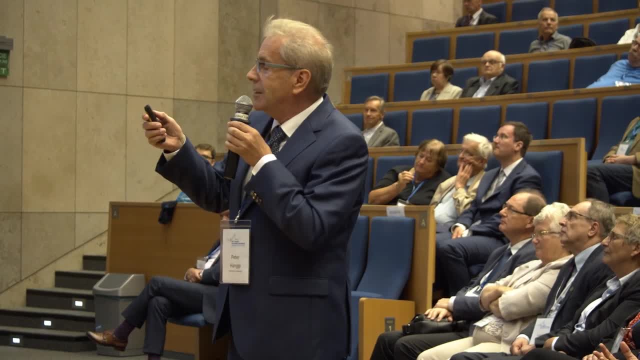 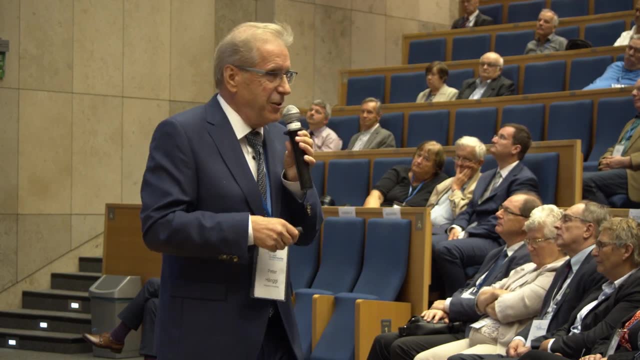 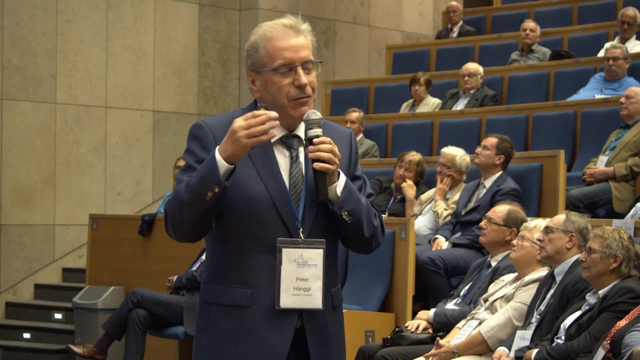 violates the second law, And the answer of Smoluchowski was that this relates to intelligence, but intelligence goes beyond the physics. That's not the field of physics intelligence. But- and this is now interesting, I say this in this audience here- he had always a way out, kind of a loophole. 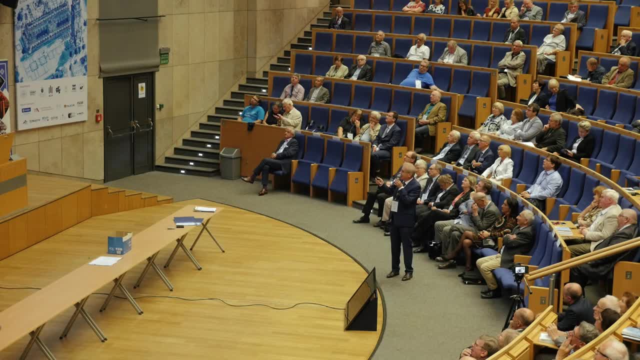 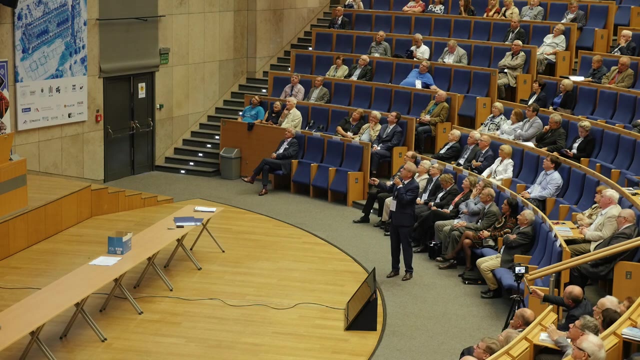 Because he continues his answers saying here- and I have to read it loud: it seemingly cannot seem excluded. Sorry, It cannot seem excluded. That's important, That sentence. sorry, sorry, sorry. This is an important sentence, Smoluchowski 1912.. 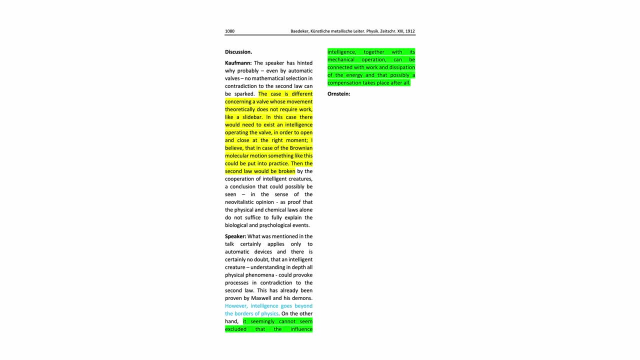 Seemingly cannot seem excluded. That's, the influence of intelligence, together with its mechanical operation connected with work and dissipation of energy, lead to a possible compensation, and that takes place after all, and you don't get the steady motion. 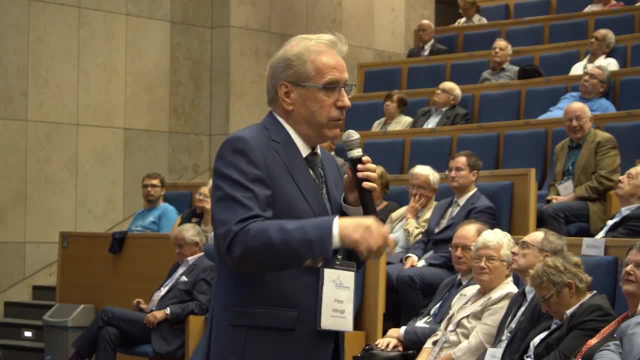 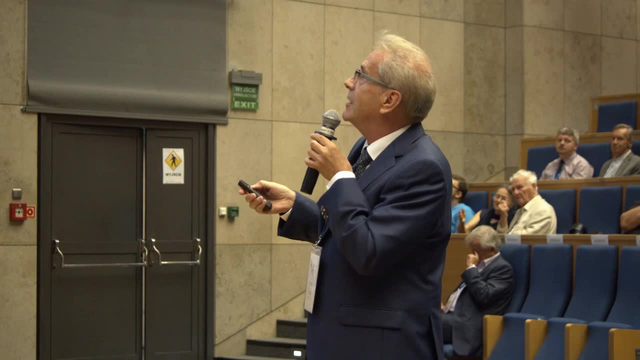 Nowadays we know a lot about neuroscience and we also know that we have to pay for everything. when you do get out work and heat, you have to actually also pay for it. So this goes back. I like that very much, I must say. I like that very much. 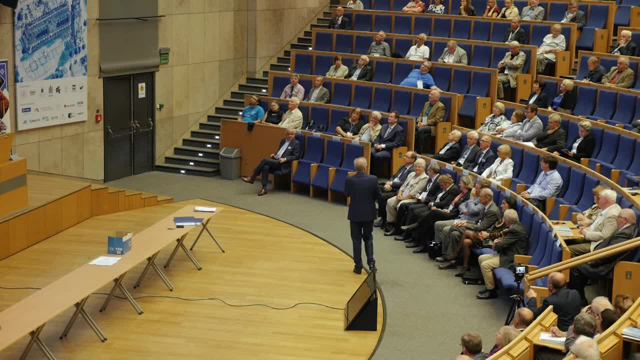 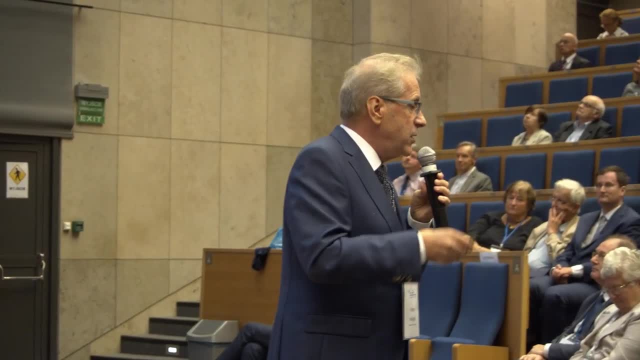 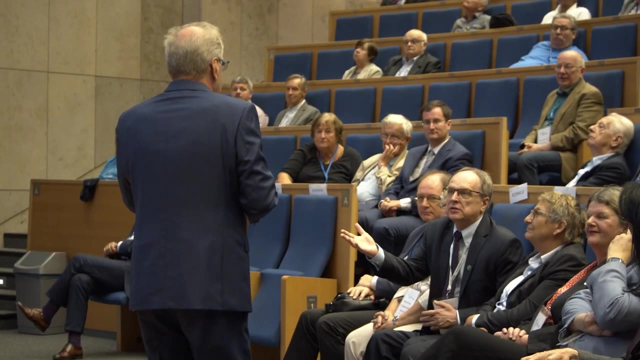 How much time do I have left? Where is my chairman here? OK, so I will actually tell you now the modern language how we get motion out. but we have to break symmetries. You are my chairman now. How much time is left for the coffee break? 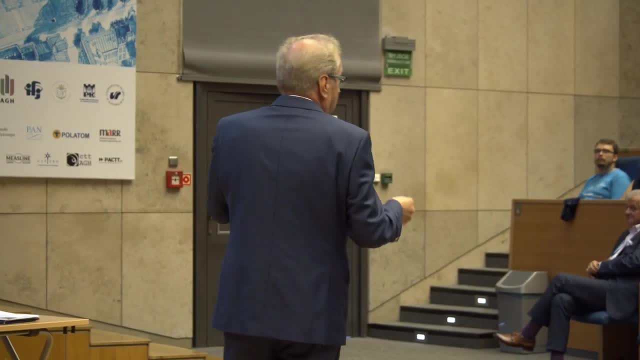 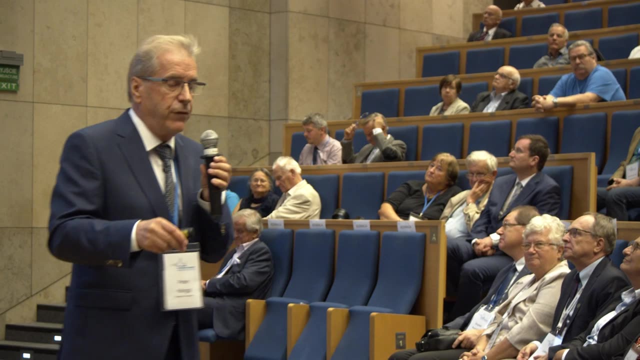 Five or 10 minutes, OK. So let me advertise this, Because we have to break symmetries, we have to break the balance, and then we're not anymore restricted to the second law, because the second law is a problem which a symmetry, a 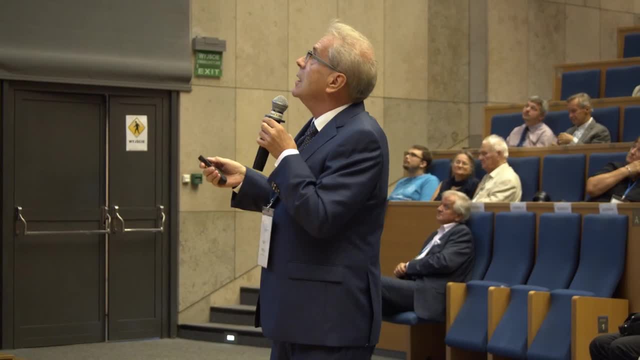 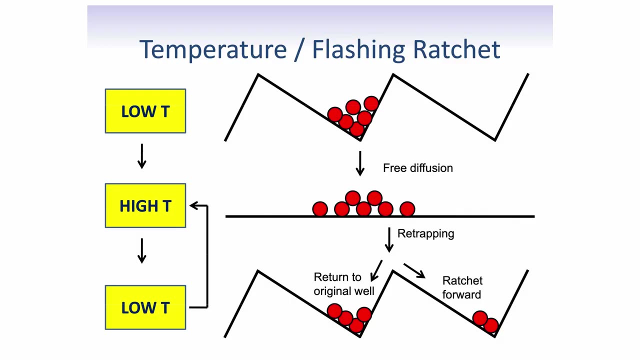 balance and if you break it, then things change. And of course here I give you the idea of a temperature or flashing ratchet. Assume you have a zig-zag potential here and you have particles located here. Now you heat it up as a function of time, periodically. 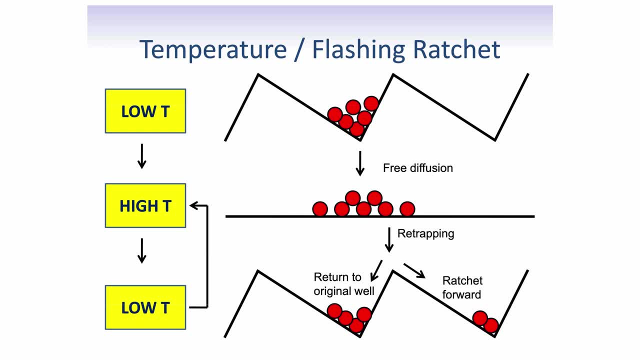 to high temperatures. So then the barrier energies are going to change. These energies at the high end, at the high temperature, are so small that you can neglect them And you get here free Brownian motion, so to speak. Now you see that this distance for this particle to diffuse, 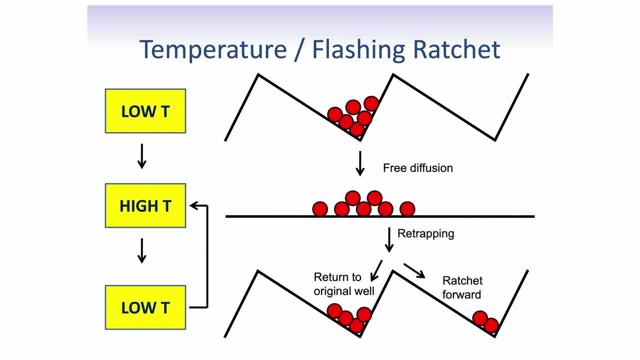 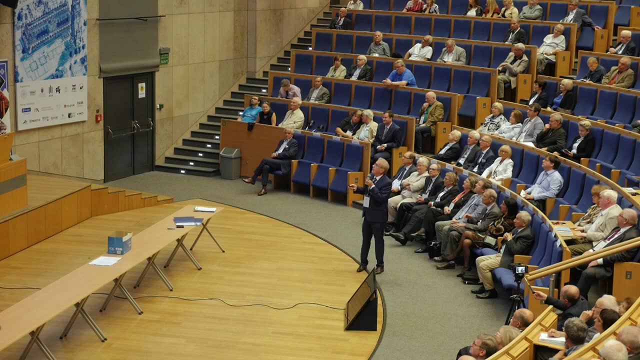 over a short distance from here to here, compared to the time it takes to travel from here to the long distance here will be much less likely. So if you do this periodically you get essentially forward motion And you can also do this. 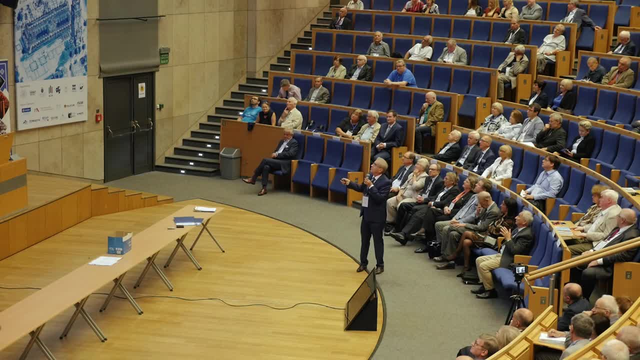 So flashing instead of heating, you just switch off the potential when there's no potential present, when you switch back the potential, which is actually used now in several experiments, also to flatten surfaces, and when, of course, you trap again. 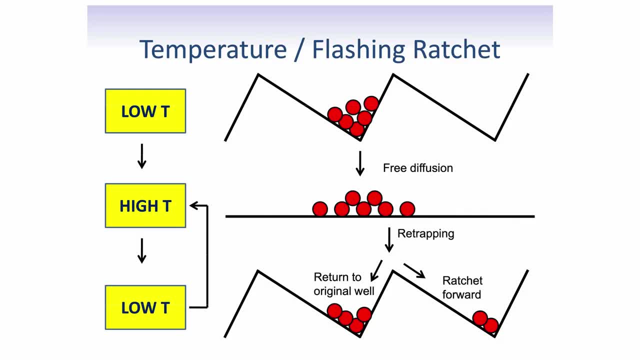 On off. on is the same as low temperature, high temperature, low temperature. And then of course you get the motion, a directed motion to the right of impurities and things like that, And this works. but remember, switching on, switching off is. 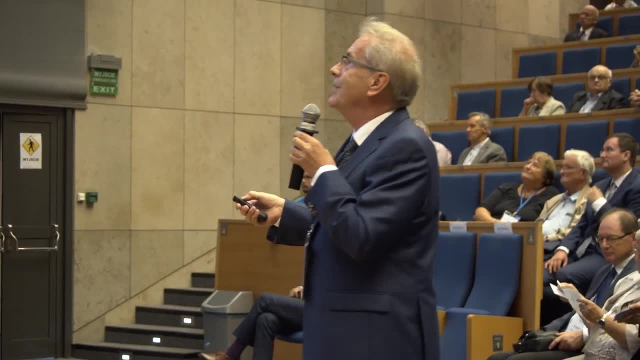 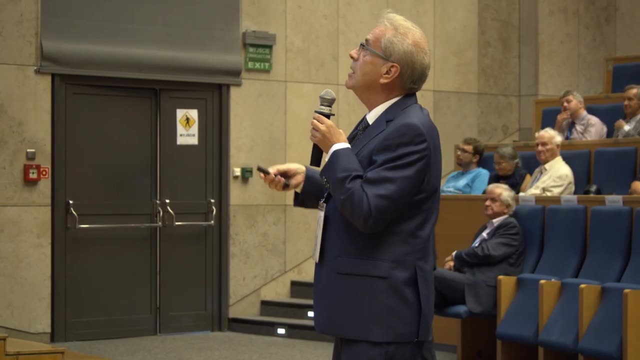 non-equilibrium. You have to pay. it costs money to do this, And that's why you have to. the efficiency has nothing to do with the second law. Now, here you see, after you move right, you can also move upwards like that with this mechanism. 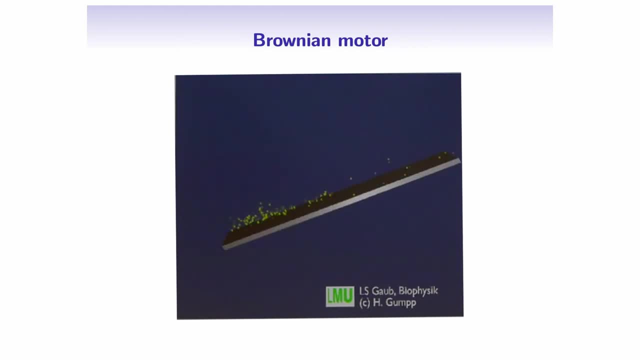 And this is an important, an important parameter, how steep you can go upwards against the hill, And this is called the stopping force, and this is actually how one measures an important character of molecular motors which take place all the time in your body, right now, as a 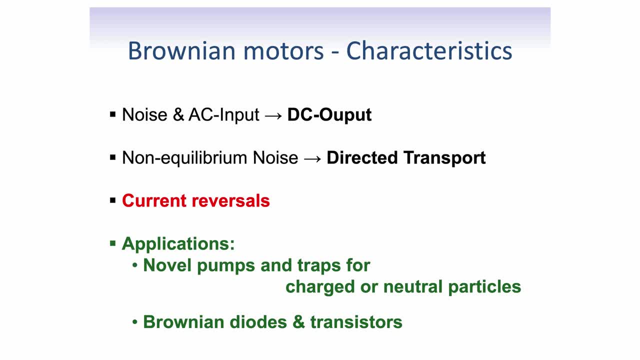 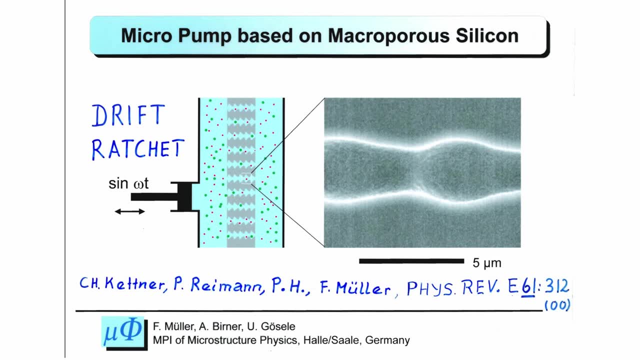 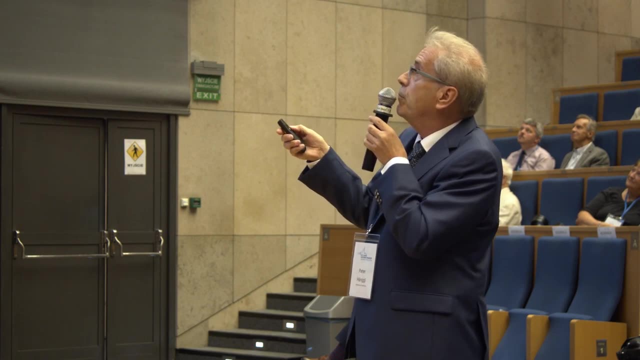 speech. OK, so this is essentially one thing We have done here. another pattern: They may want to move with this effect, infected cells, which are usually bigger than healthy cells, using hydrodynamics and hydrodynamic interaction by pumping forth and back here. 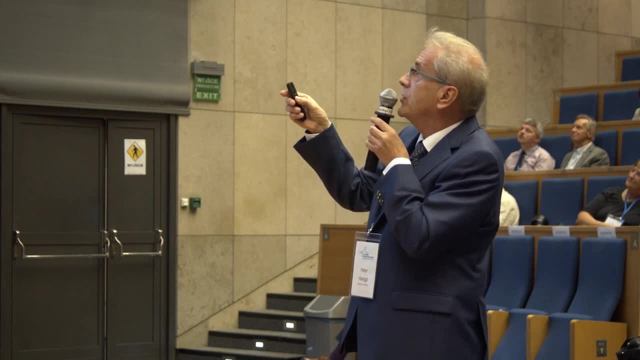 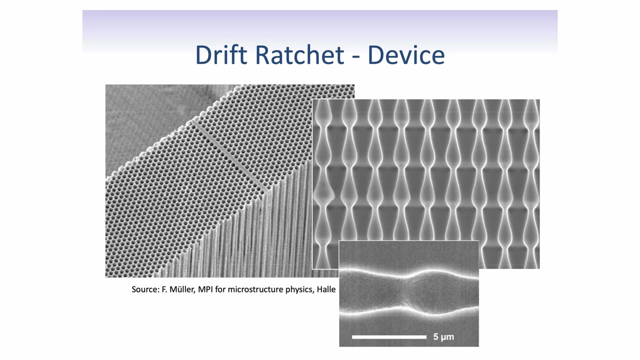 This is pores of about 10 million pores which are asymmetric, as you see, on the square centimeters, and there are experiments. as I say, that's a length case. there's a micrometer stuff of motion and we have 10,000 pores. 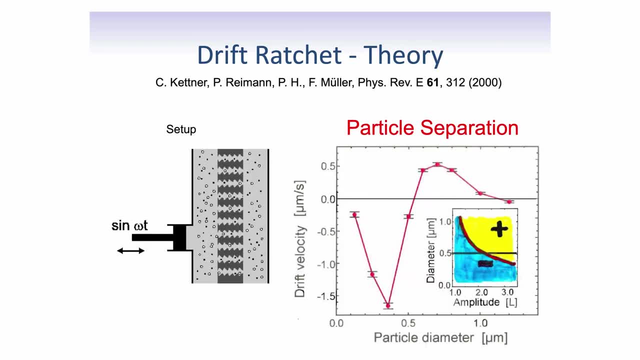 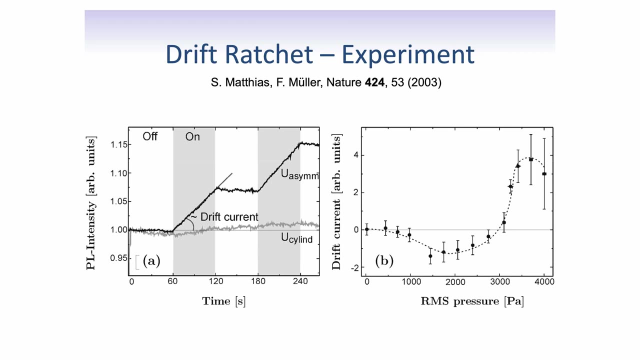 10 million pores per centimeter squares, And this is our calculation. you can pump the particles depending on the diameter, either going left or right, And here is the experiment in nature, without going into details, where you can actually switch off the pumping, you get. 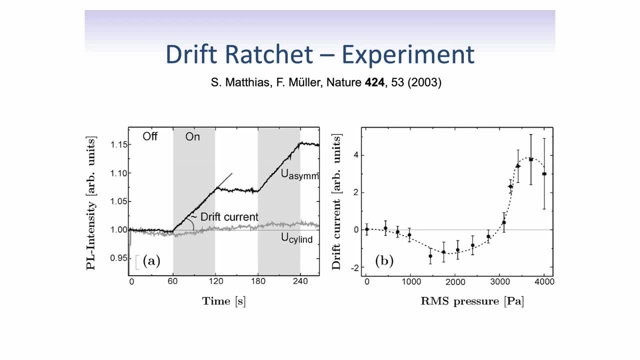 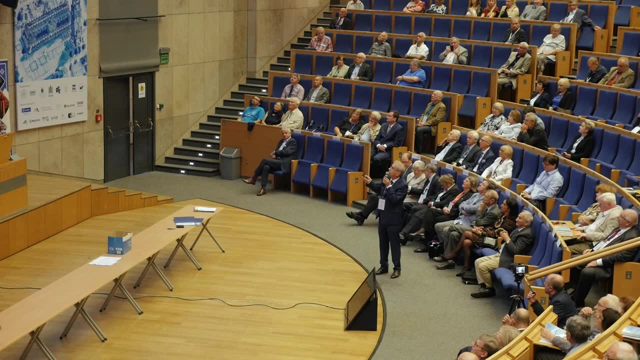 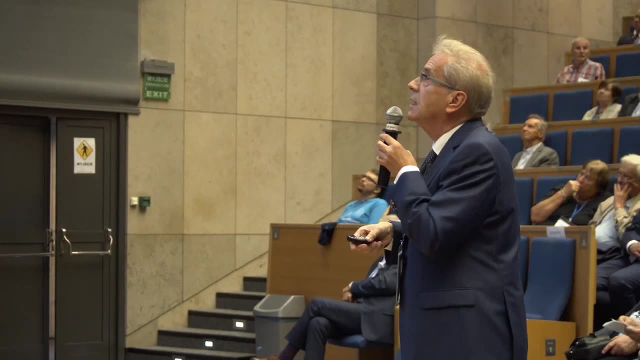 no drift. switching on the pumping, you get the drift, And that's how you can separate the infected cells from the healthy cells without using chemical means. I have a little bit to say, something in my last two, three minutes, about quantum mechanics, namely quantum. 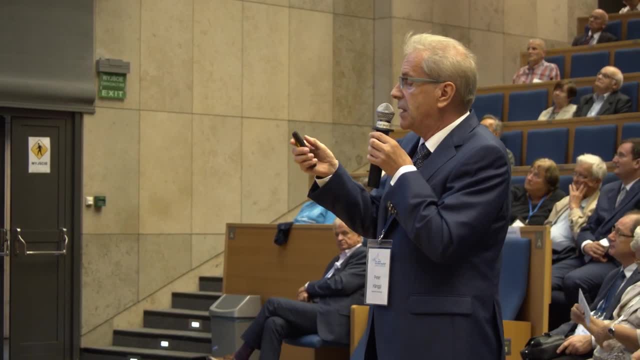 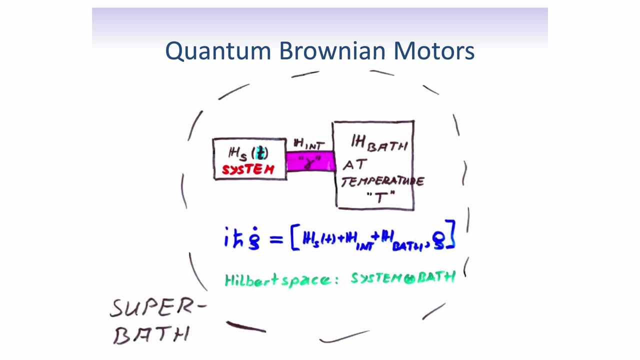 mechanics. to do this on the quantum mechanical level is quite complicated because you have to treat dissipation and there's no phenomenological law on the system space where you can treat dissipation. The problem with quantum mechanics is that you have always to go to the Hilbert space of the system, the Hilbert 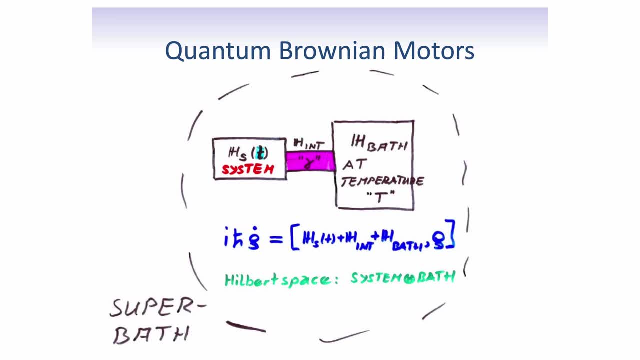 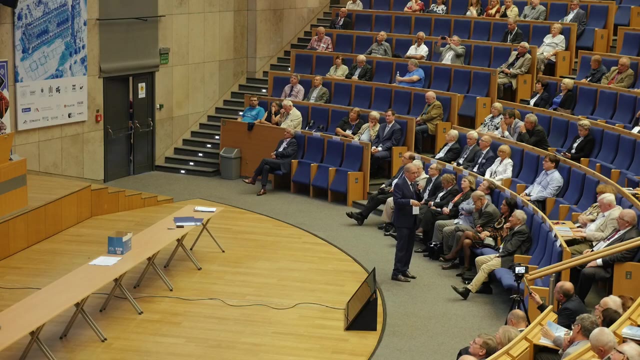 space of the path, which is usually infinite, and the interaction And, of course. so if you integrate out the path, you still have, of course, the fluctuating forces which are operating in the path. Hilbert space. This is much more complicated than in classical, where the 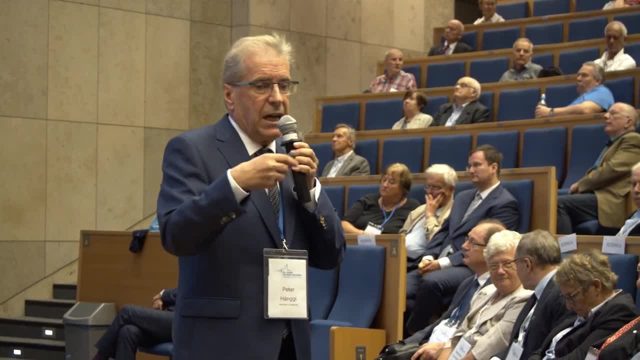 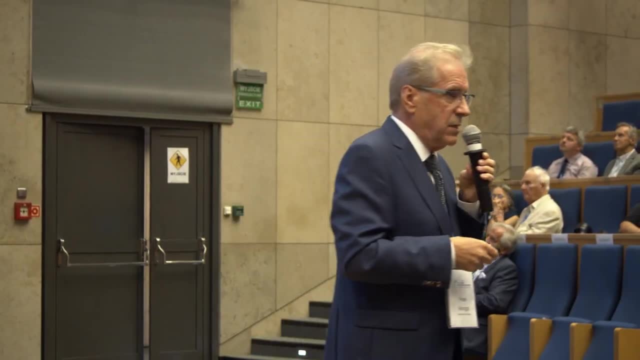 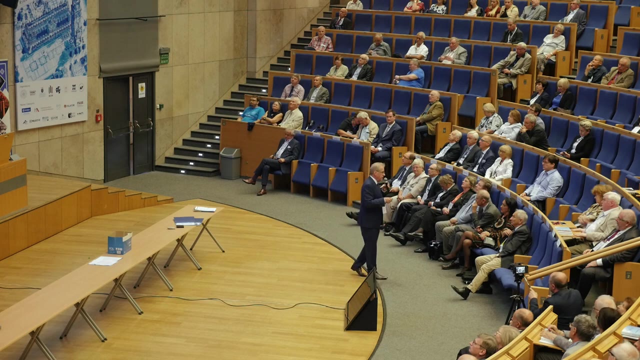 stochastic force is a classical force which is essentially acting on yourself. This is much more complicated than in classical, which is essentially acting on yourself. And then you have the. So that's why a lot of sense and nonsense is being published in quantum thermodynamics, in particular about heat. 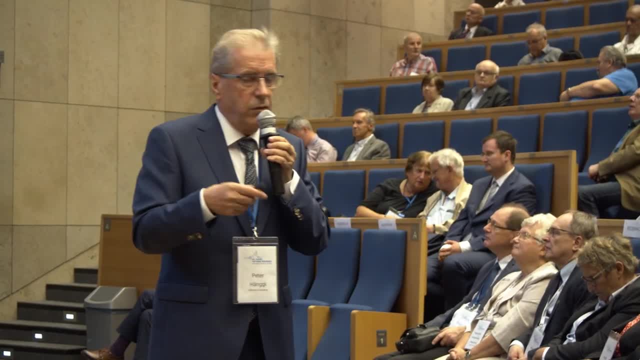 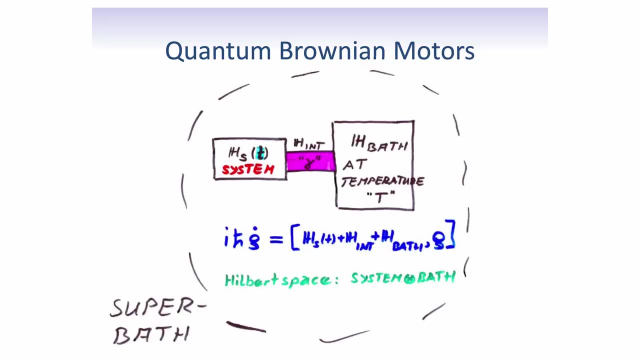 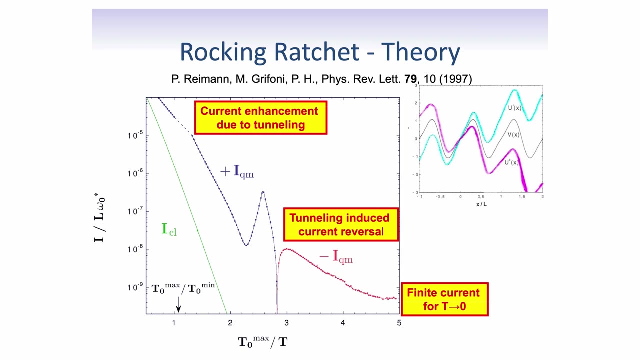 Because I have a theory that heat and quantum mechanics cannot be defined, but work can be defined. But of course heat is given as a difference of internal energy and work And when you have the problem, heat depends on how you define where quantum ratchets have been done and this is get new effects because of 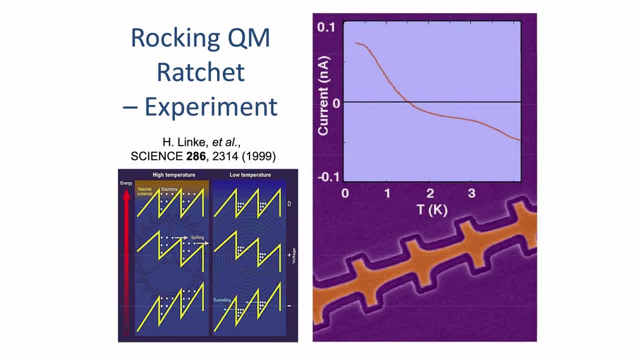 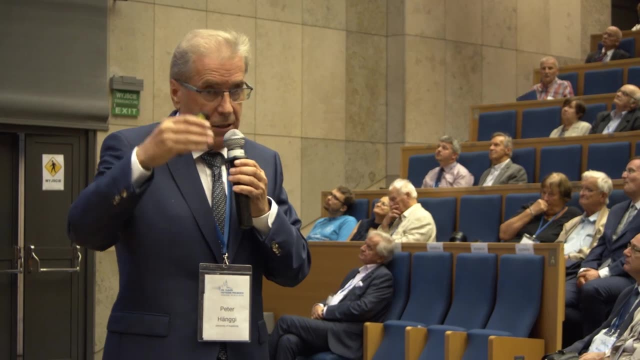 quantum tunneling. you see here, when you tilt the classical ratchet you get always positive currents to the right in adiabatic limit. but if you tilt a quantum ratchet at low temperatures now you get a battle between thermal activation means high barrier paths, low barrier at low temperature you have high. 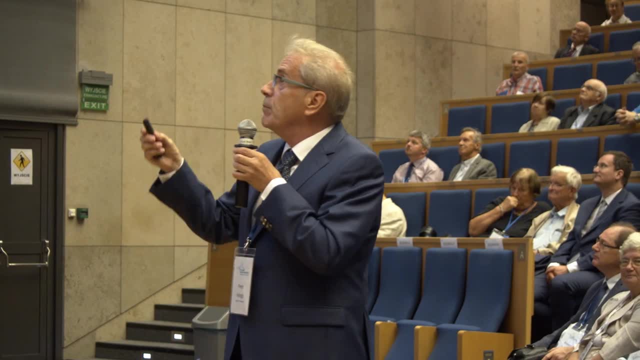 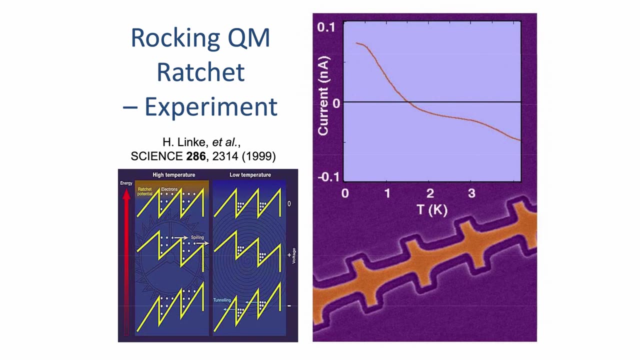 barrier. it's a big array factor. it's a battle, it's not good, but what helps you is not only from the gamma factor, not only the height, but also the thickness of the barrier, and if you tilt to the left, the thickness of the barriers are smaller as compared if you tilt to the right, and this gives you then a current 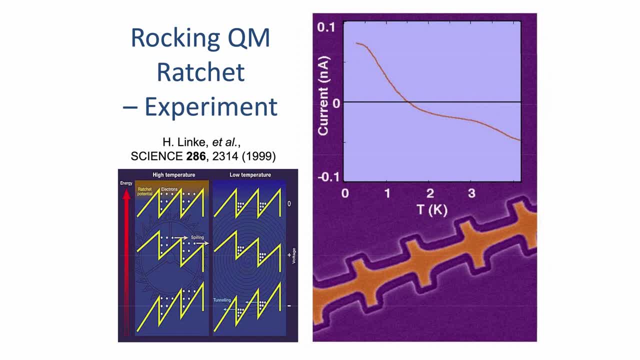 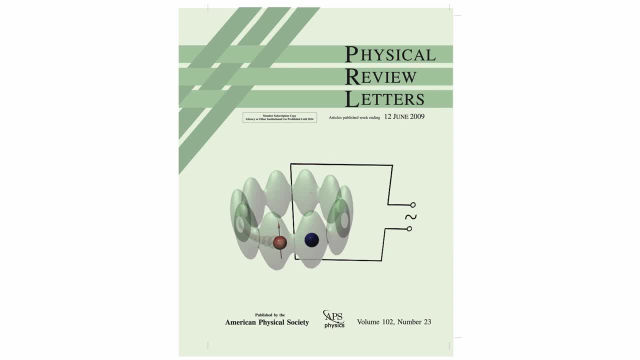 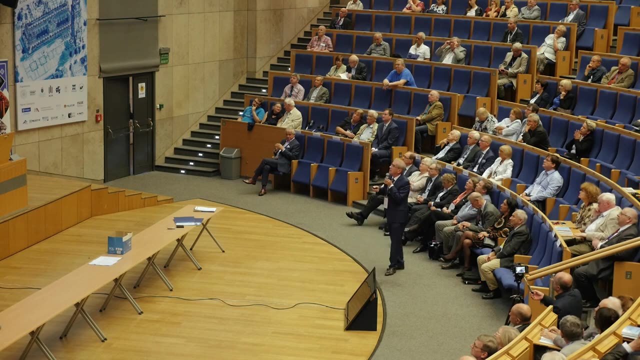 reversal which is solely, rigorously induced by quantum tunneling. okay, this I have no time you can have also ratchets without dissipation with. this relates to the field of floquet crystals, how to drive coherently systems and how to actually what to do in order to get direct current on such things. 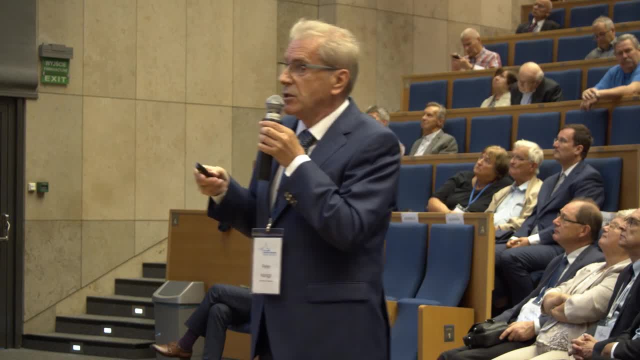 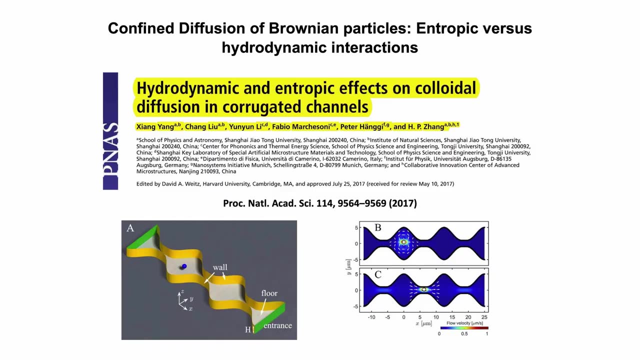 here, like on this ring, and of course there are modern directions where you treat active particles or Brownian motion on the confinement, and then of course the big problem is that one has to take here hydrodynamics into account. here you see, you have a narrow position, you have a wide position. 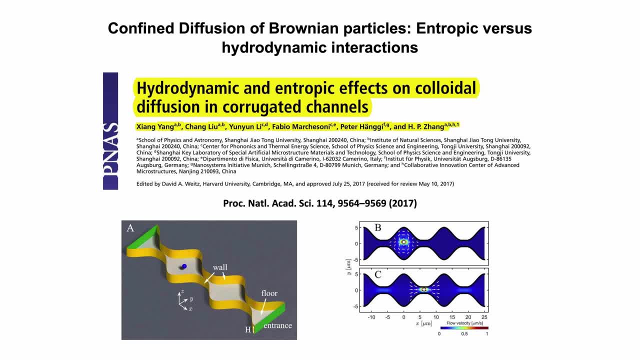 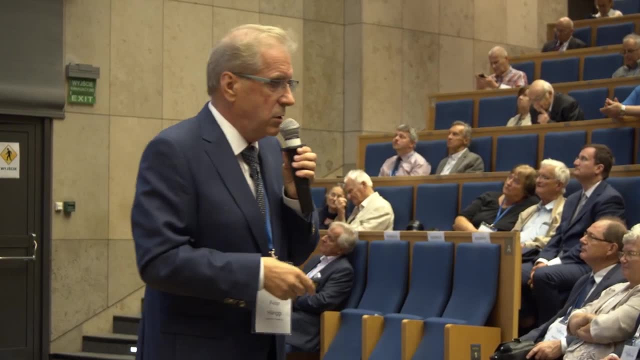 and the hydrodynamics around here is much more. it's much more simple than the hydrodynamics here, where you have so to spoke friction laws, but also hydrodynamic on scene type interaction and hydrodynamics wall interaction. that's something I do with the people in Shanghai and TTL Institute and see. 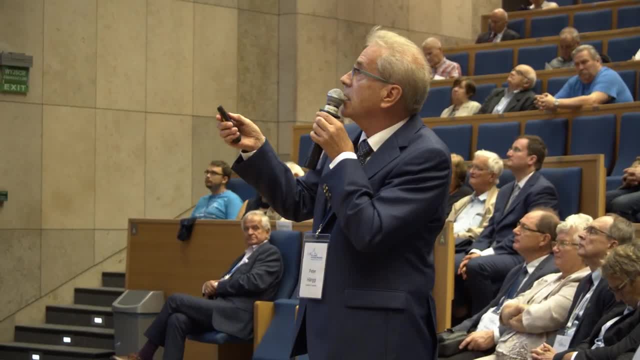 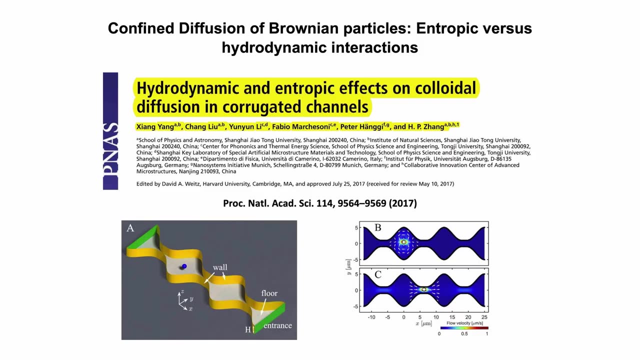 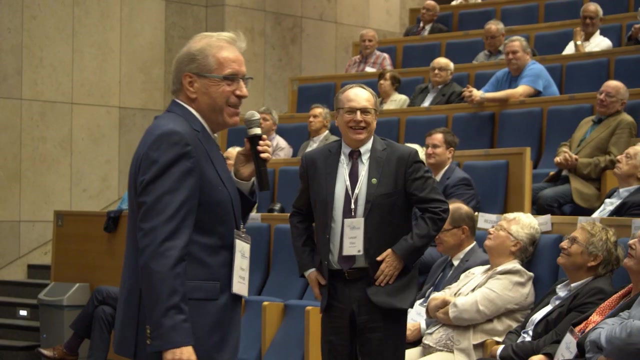 Shanghai Jia Tong University. this is a paper recently from proceed International Academy, where's the effect of hydrodynamics is up to 200%, as if you would neglect it. so, coming to my end, I am in time? of course not, but I want coffee. yeah, yeah.